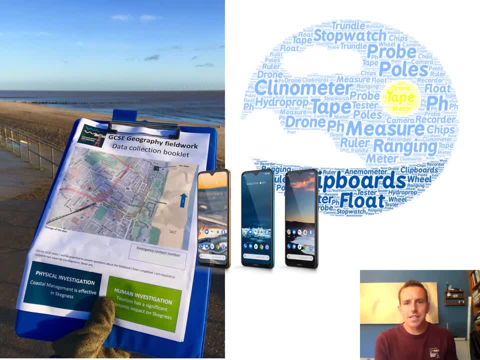 making lots of grids, making questionnaires and surveys, putting them onto A4 pieces of paper, maybe sometimes, if you're lucky- stapling those together to make a little booklet and then having a clipboard that you use to lean on and going out and collecting all of your data on these. 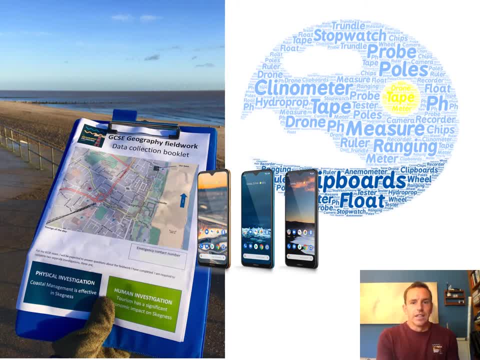 homemade booklets, I suppose, and that's absolutely fantastic, That's absolutely fine, and there is definitely still a place for using clipboards and booklets in geography. but very often people perhaps don't consider using the technology that you've got in your pocket and most of you will probably have access to a smartphone or a mobile phone of some type. 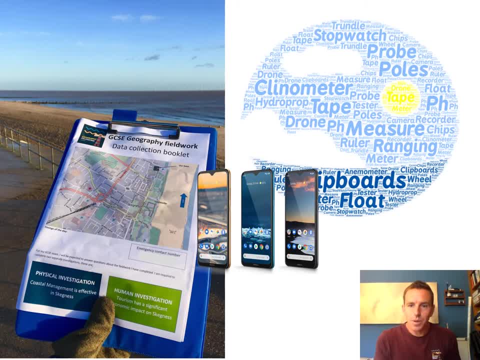 and the power and technology within those devices that we have in our pockets are huge, and when you compare that to the power and technology of a piece of paper and a pen, then sometimes it's like chalk and cheese, and I think now is the time really for us to, rather than 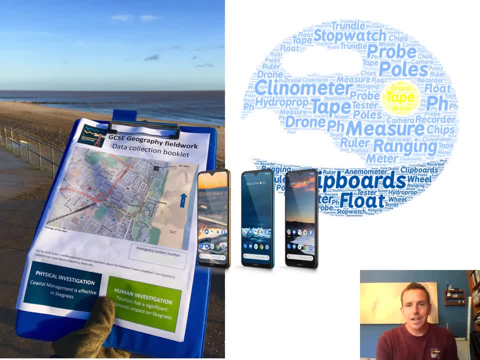 being, you know, afraid of the technology that exists in the 21st century, then, for fieldwork in particular, we need to embrace it and it can create huge opportunities, and it can give us the opportunities to not only help with our data collection but definitely help create more modern and better. 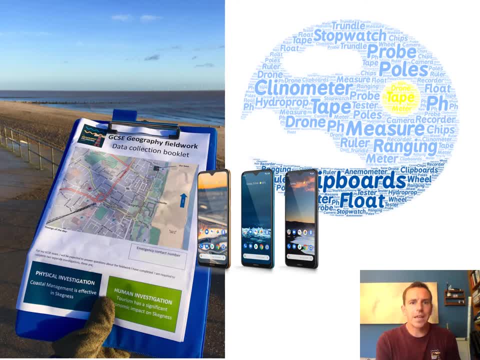 frankly, forms of data presentation. So in this session, I'm going to talk a bit more about using technology in your fieldwork and give you a bit more of an idea about how you can do that, but also a bit more of an idea about why you should do that as well and why using technology can create better fieldwork projects. 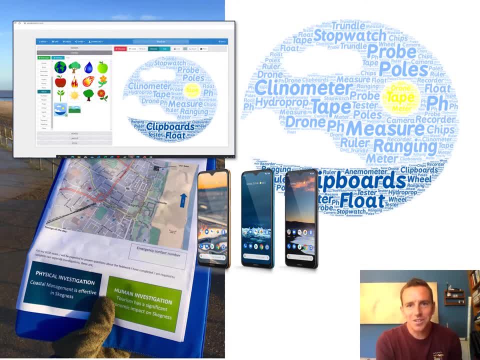 So, just while I'm on this screen, I thought I'd just highlight to you this thing on the right hand side of the page. this is something that I'm sure you've seen before. it's called a word cloud, and I wanted to make a word cloud just to show some of the different geographical equipment that we use. 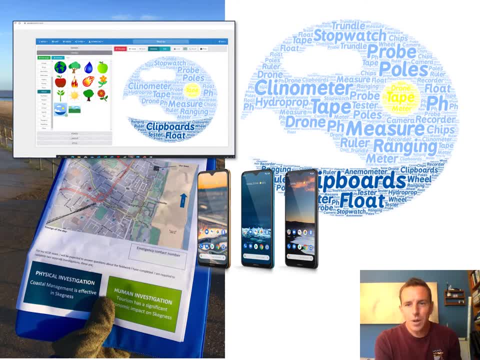 on our fieldwork courses and I went on to Wordallnet, which is the one that I normally use for creating word clouds, and that's great. but actually there's a few other ones and I found this one which is called WordArt, and WordArt allows you to create word clouds, but 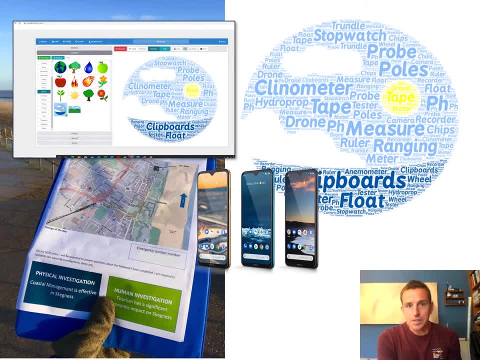 actually in the shape of different bits of kind of custom art that are on this website. so it's just a nice website I came across. I thought you might, if you have got this kind of qualitative data, might be interested to have a look at it. it's free and it allows you to create nice little word clouds. so 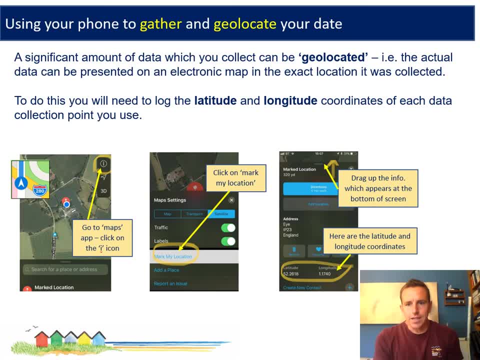 there you go, WordArt. take a look at it if you need to. Okay, so firstly, first thing that I want to just go over with you folks is that one of the things that smartphones can do is they can obviously use satellites and GPS and they can track your position and they can tell you at any point where you're going to be on your fieldwork. 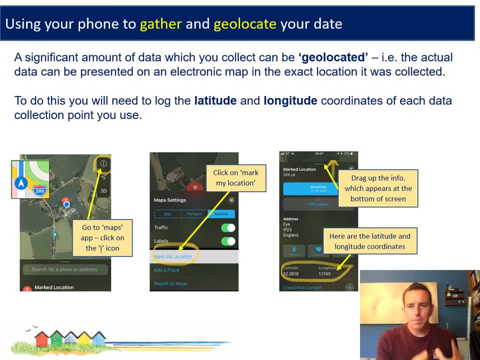 You are where your phone is and your phone has got the ability to gather detailed coordinates, or latitude and longitude coordinates, and if you can take those coordinates off your phone, then you can use those numbers to help you present what's called geolocated data. so, rather than 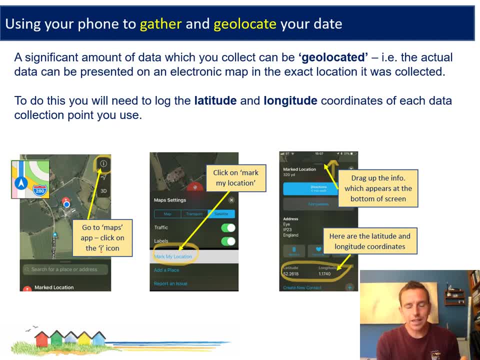 perhaps doing traditional fieldwork. let's take again, for instance, the example of the pedestrian count. it might be that you go to a town and you select 10 streets, you write down the name of the streets and you do a pedestrian count, and then you might then be able to present how those 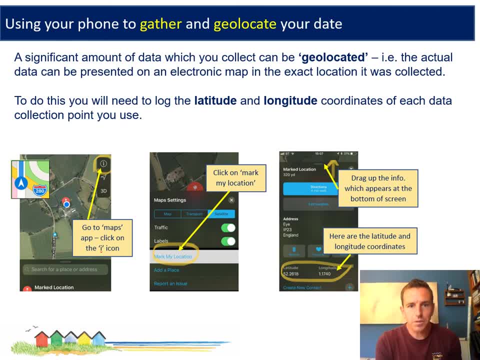 pedestrian figures vary, and by doing a bar chart, for instance, and labeling each of those bars the names of the streets that you went and visited, which is fine, but it's a bit basic and it's not bringing your fieldwork to life. so, actually, if, instead of get when you're on that street instead, 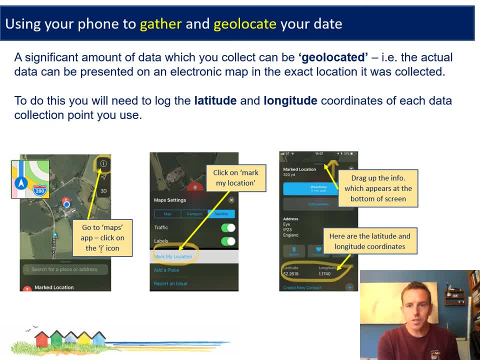 of actually getting the name of the street, if you instead got the coordinates of where you were standing when you recorded that data. What you'd then be able to do is use that data later on, using a website which I'm about to show you, to actually plot physically on the exact location of the of a map where you gathered. 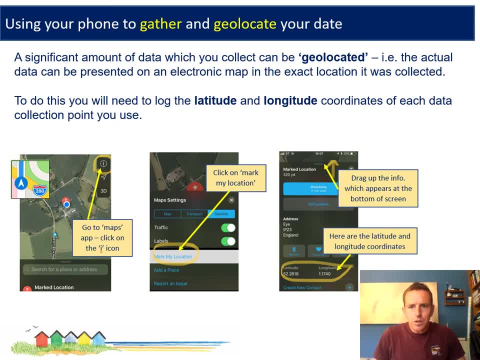 that data so you can actually see the distribution of your fieldwork data at a glance by looking at a map and seeing how your numbers and your figures vary across that given map or location that you're using. I might not have explained that very clearly, so I'll go on through a number of other. 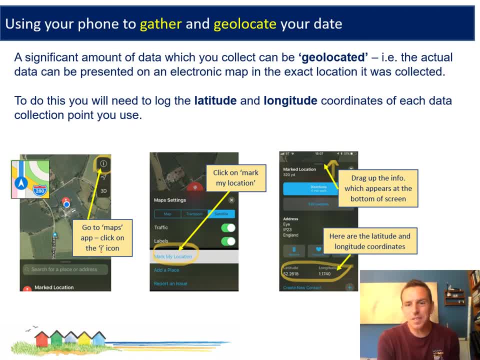 examples just to make that clear, because at this point you might be thinking I'm not really interested in geolocated data and GIS and things like that. I don't really see the point and that's fine. and I would say I've been on a number of different courses for learning GIS skills and 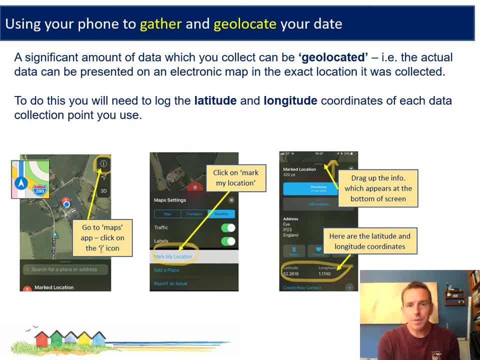 very often on those courses. it can be a bit overwhelming, it can be a bit bamboozled by all the technology, and actually a lot of the technology that we can use as students to create GIS maps haven't actually been designed for students and are not all. 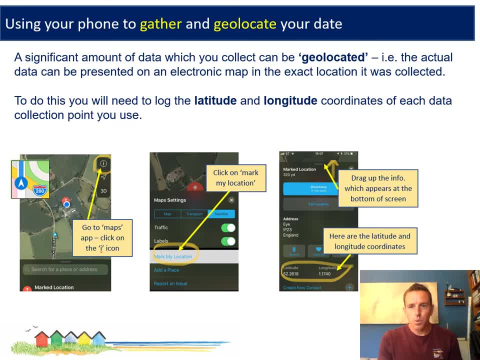 ways that student-friendly, and so sometimes I think it's important just to kind of pick out the basics and just try and grasp the basics of making a simple GIS map, which is what I'm going to try and do with you guys now, because it is actually, if you just stick to the basics, a very straightforward. 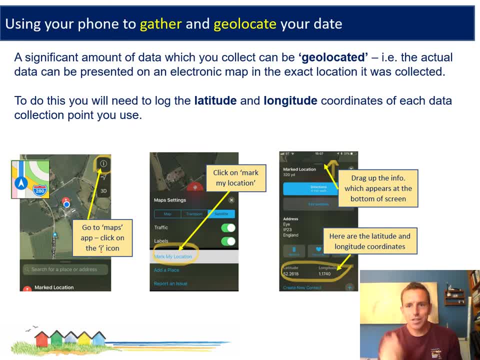 thing to do and you will be able to, within the next 15 minutes, to be able to produce your own GIS map, and those look great in NEAs. they're high level bits of presentation and they're well worth sticking with as I go through this explanation, even if I've not started all that clearly. 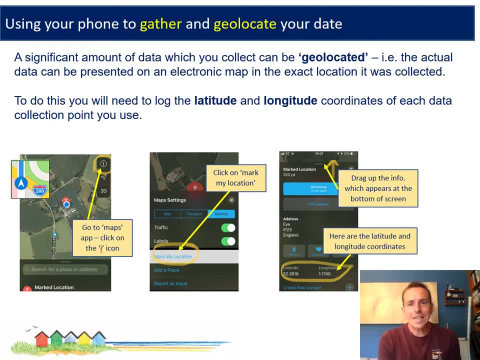 so the first thing that I would like you to do with your phone is to try and work out how you gather the latitude and longitude coordinates off your phone. now, the example that I've got on the screen here is for an iPhone, and that's getting your latitude and coordinates off Google. 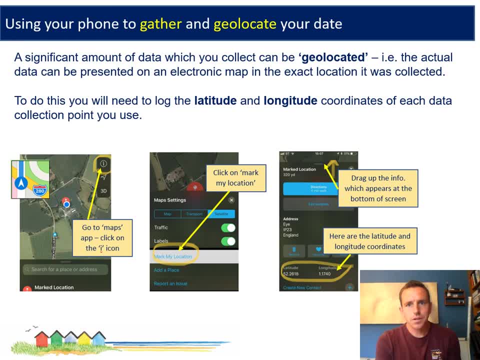 Maps. but if you just type into Google, how do I get latitude and longitude off my phone? it would be slightly different, probably for an Android and an iPhone, and perhaps slightly different depending on what map setting you're using. I think actually there's a few apps that allow you just to get. 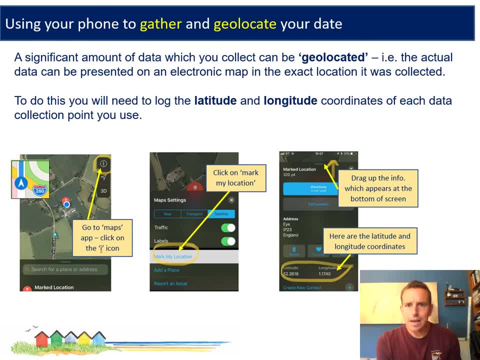 your latitude and longitude. I think some iPhones have got a compass app that are already kind of designed into it, so just take a few minutes and see if you can work that out. it is possible, so just persevere until you can get it. but your latitude number is normally. 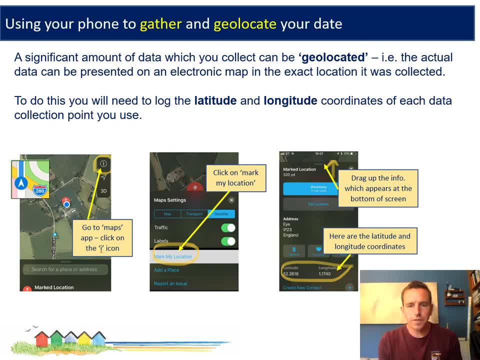 the one that comes first and is normally 52 or 53 or 51 point something. and your longitude number is the one that comes second and is normally one point something. generally for ArcGIS you could gather maybe up to four or five decimal points. you don't necessarily need to write down. 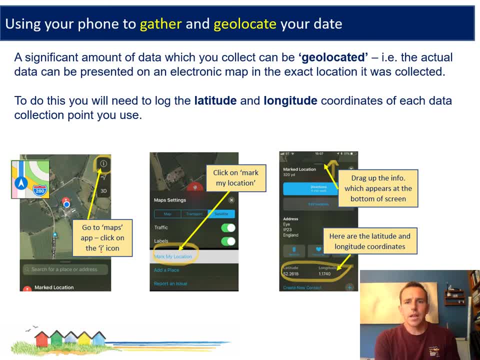 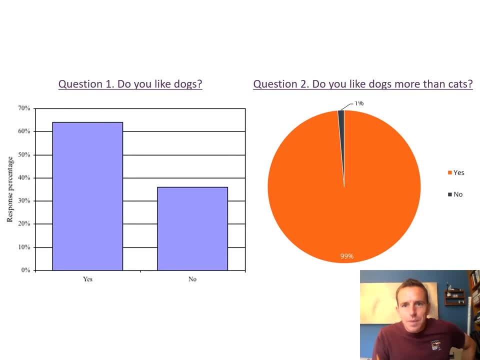 seven or eight or nine decimal points. four or five is fine. so the reason that we're starting to think about this idea of using geolocated data is because, essentially, it gives us the opportunity to make better quality data presentation and very often when students have done field work previously at GCSE or at key stage three. 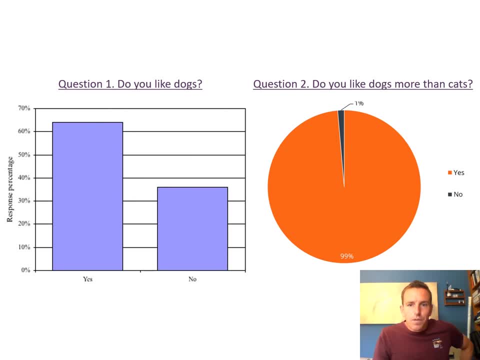 and they've been told to present their data, they very often default to the same formats, whether it's a pie chart or a bar graph, or sometimes a corridor map and or line graphs, for instance. these are fine, but there are different ways of presenting your data in perhaps a more engaging format, and that's the purpose of- well, not the purpose, but it's one of. 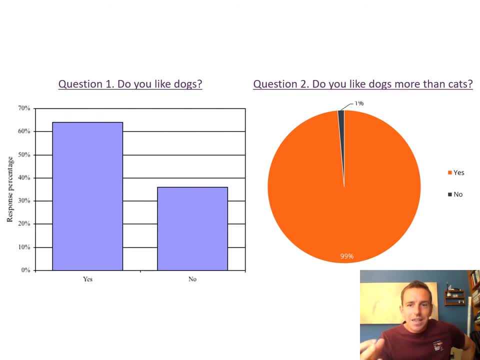 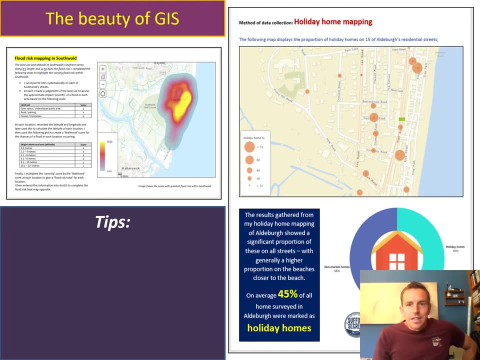 the benefits of GIS is that you can make your data much more relevant by showing where you collected that data from, so on the screen. here I've got a couple of examples of GIS, which has been homemade by students and looks really modern, really engaging and, crucially, shows the data that. 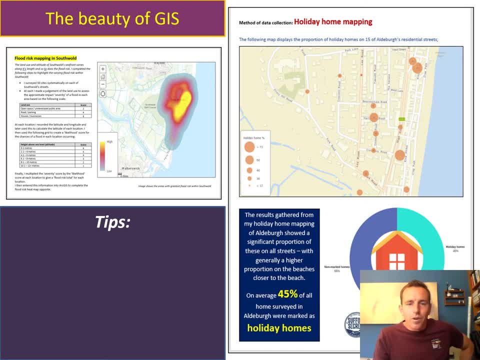 students have gathered in the exact location where they gathered it from, and those do look advanced. I I would say They're bits of presentation that would definitely impress an examiner. They would impress me if I saw those and I'd say, oh, look at this, This is great. The student is using modern 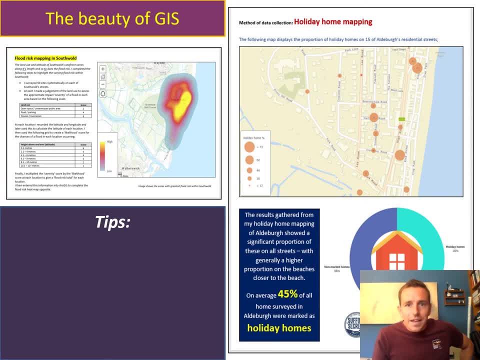 technology and presenting their data in a modern format that's really visual and clear and beneficial and, you know, impressive. And it's colourful as well, which is nice. So using your phone to gather the latitude and longitude of where you're gathering your data is really useful. 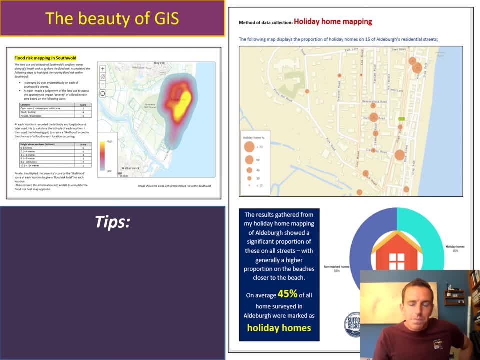 because it will allow you to create your own GIS maps, And this is what I'm going to show you how to do in a second. So a couple of tips. Your presentation, I would say your presentation section in your studies, should look good. They should look appealing, accessible, engaging to. 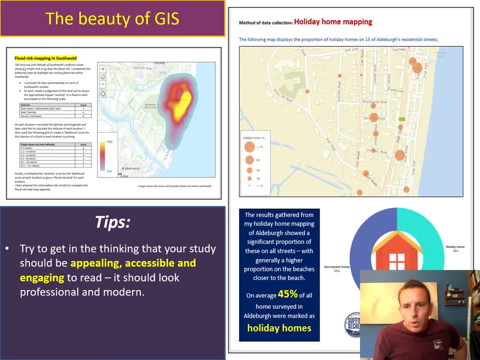 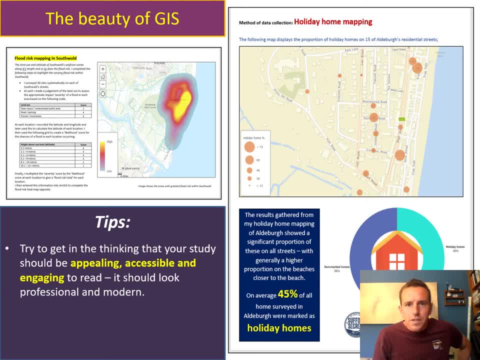 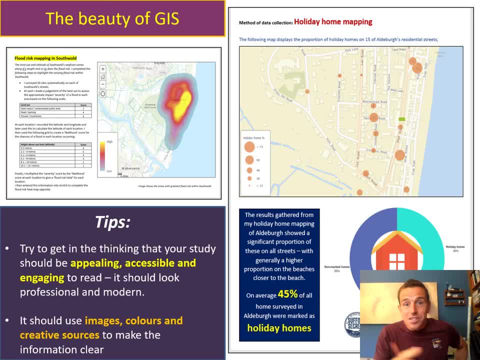 is a section where you can include colour and creative sources, And it doesn't just have to be GIS maps like this, but there can be other sources of information, like infographics, which I'll touch on later, which can help engage the reader and also help present the data that 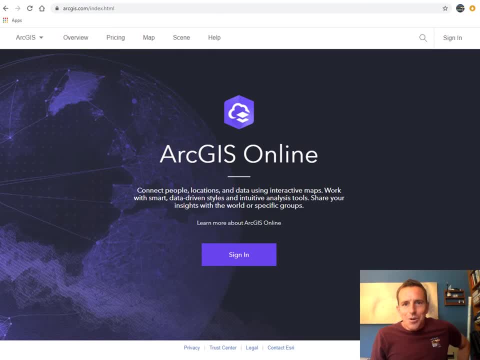 you're looking for, And then there's also a section where you can include the data that you want to use in the classroom format. So, to start off with what I'm going to introduce you to is this website here called ArcGIS online, And this is a beast. It's a fantastic tool. ArcGIS is an incredible. 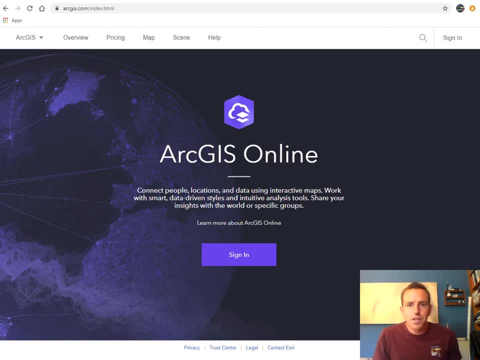 resource that's not just available to teachers and to students, but lots of anyone essentially. And when you search for ArcGIS, this is the result that you get. You click on Google. this will take you to ArcGIS. It kind of almost draws you into signing up to it, And you can sign up to it And 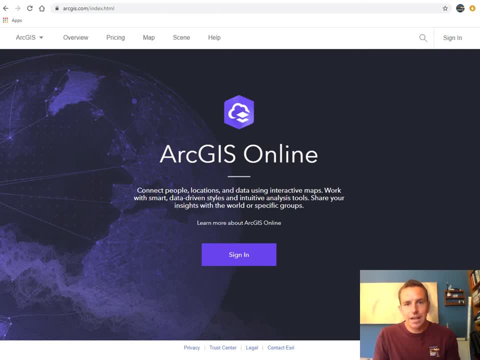 perhaps a number of you will already be signed up with an account to ArcGIS And if you have that, by all means log in. But it isn't an essential. You don't have to sign up to it and you don't have. 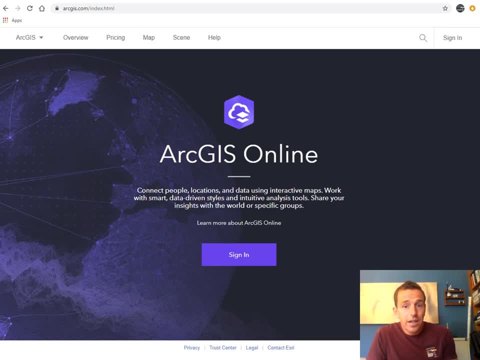 to commit to having an account. It's free at the moment, I think, But I would suggest that the easiest thing for you guys to do for what you need to do and getting started the basics of ArcGIS- is just simply to click on. 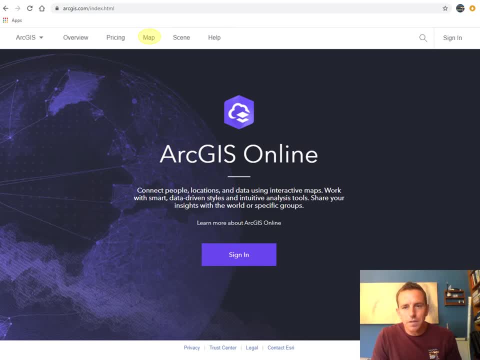 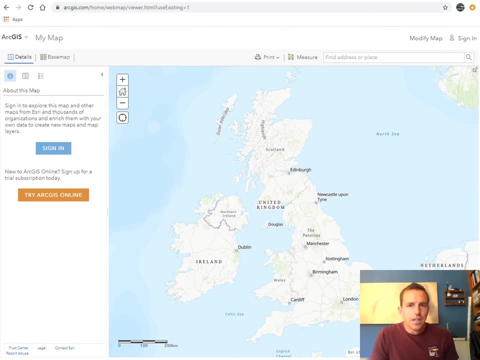 The map word up there on the top kind of toolbar. If you click on that View to this page- And this page here is essentially the start page for getting ready, getting started with ArcGIS- And it will default, if you're in the UK, to a map of the UK like this: 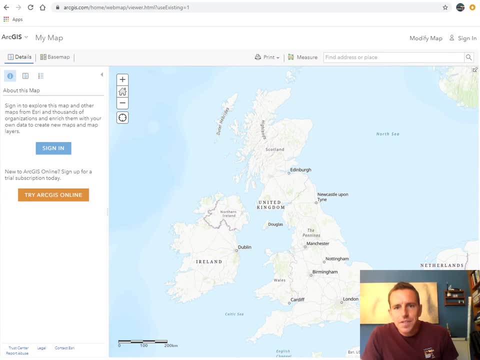 And at the moment that map is looking a bit empty of data And it's got, obviously, a few towns and cities dotted around it And it's got the name of our oceans and seas, But it hasn't got any specific data that need that is being represented. 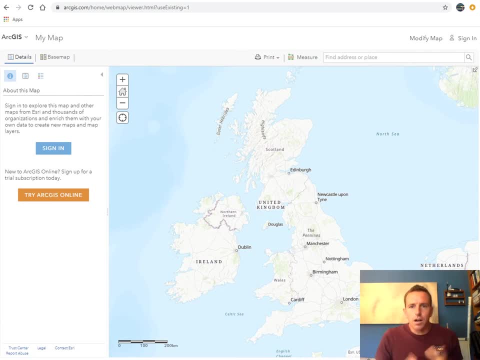 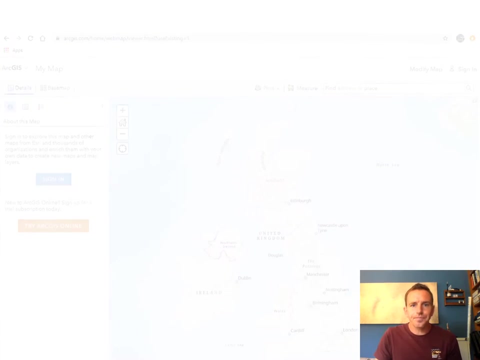 on it. So at the moment it's a bit of a blank And our job is to feed that map with our data. And if we give that map our information, then it will present the data that we give it in the exact location that we collected that data. So here's how you do that. First of all, using your phone. 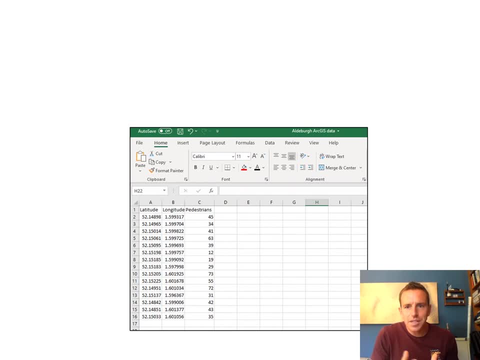 you can collect the latitude and longitude of every single bit of data that you gather And that, for instance, if we're doing things like traffic counts, environmental quality surveys, pedestrian counts, that can be something that you can just write down into a list like this: 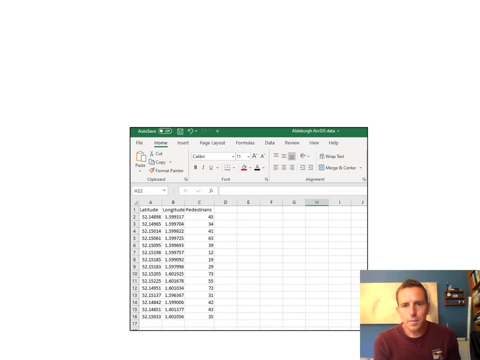 And you might have site number one. First of all, I'm going to gather my latitude and longitude for my position at site number one And then I'm going to do my survey And you can see here that, ultimately, this student has been able to go back to their computer, has. 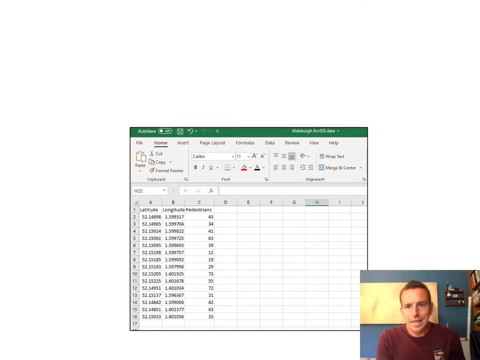 opened up Excel And in Excel then they've just made a basic template. So this is what ArcGIS wants. It wants a template like this of information In your first column heading type in the word latitude, In your second column heading type in the word longitude, And then in the third column. 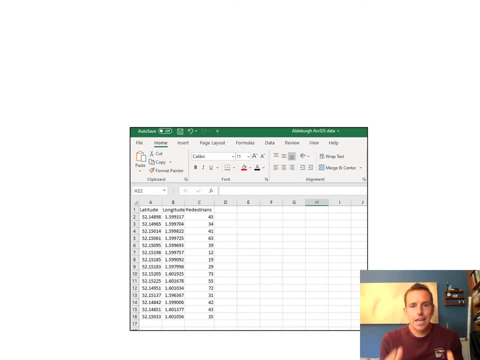 heading, just to get you started, type in the name of whatever it is that you've collected- So in this instance it's pedestrians, but that could be anything there- And then fill in that grid with the latitude and longitude and the results that you've collected, And then you can then fill in. that grid with the latitude and longitude and the results that you've collected, And then you can then fill in that grid with the latitude and longitude and the results that you've collected, And you can then fill in that grid with the latitude and longitude and the results that you've collected. 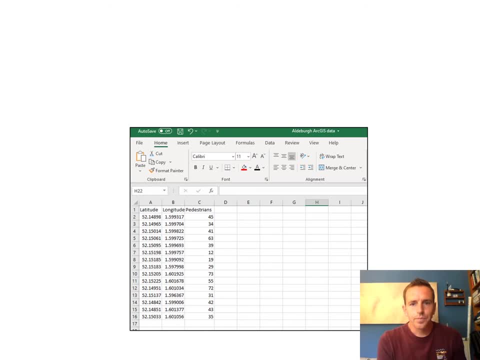 That were relevant to the field work that you've done. From this point, it's important, then, that, before you try to add this information into ArcGIS, that you save this as a file. save it somewhere that's accessible. But, importantly, when you save it, save it as a CSV file If it's not saved as a 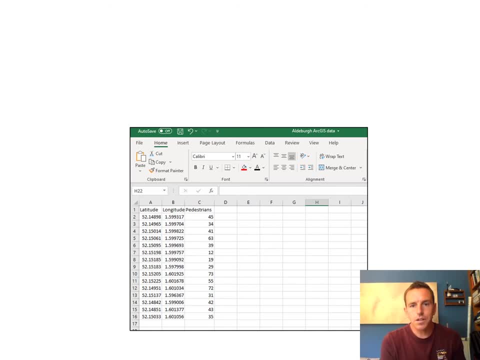 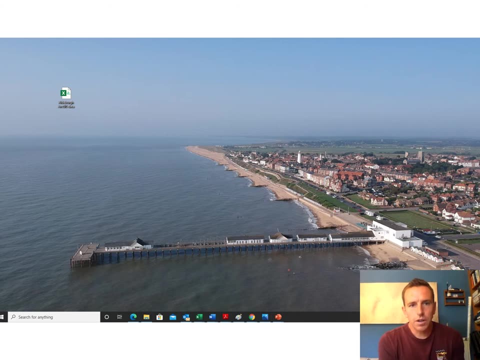 CSV file, then it won't be recognized in ArcGIS And it's just the format that ArcGIS likes. So save it as a CSV file somewhere where you can access it. So I've saved mine on my desktop And then I'm going to go back to my computer and I'm going to go back to the. 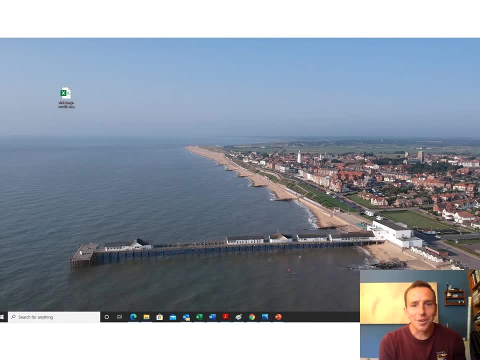 desktop here. So fairly uncluttered desktop doesn't always look like that, But I wanted to unclutter it, so it looked like that. Well, so it is clear that you could see what I mean by saving this file somewhere that's accessible. So it's on my desktop there. My next job, then, would be to 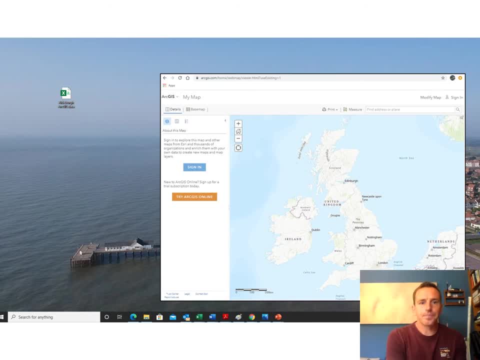 pull up ArcGIS again. So that was like that, if you remember. And then simply all I would do is I'd grab that file, drag it and drop it onto the map over here, And then I'd cross my fingers and hope that the magic happens And it does. 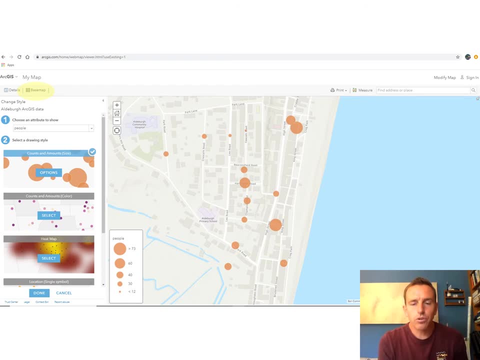 And eventually, when the page then loads, it will transfer or transform the map in front of you from a UK one to a more localized one to where you've collected your data, And you will have your data represented initially by these kind of orange colored proportional symbols. So that's the. 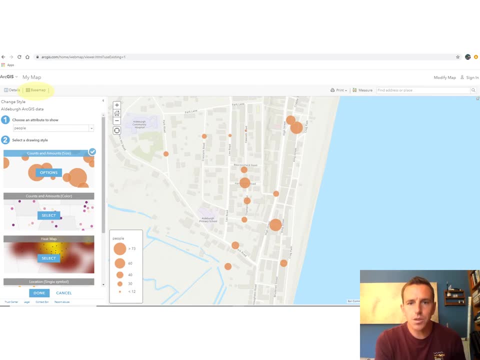 default map that ArcGIS presents your data in. But you'll see down the left hand side of the page that all of a sudden there are lots of different kind of options And those options are things that you can explore through and you'll become very comfortable with. So I'm going to go back to my 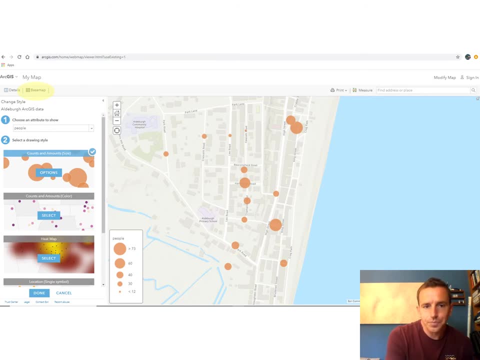 steam FTP account very quickly- Confident apps, just kind of tweaking and playing around with those- And you can change the color of those proportional symbols. You can change the shape at those symbols. You can click on the heat map section and turn it into a heat map, which is: 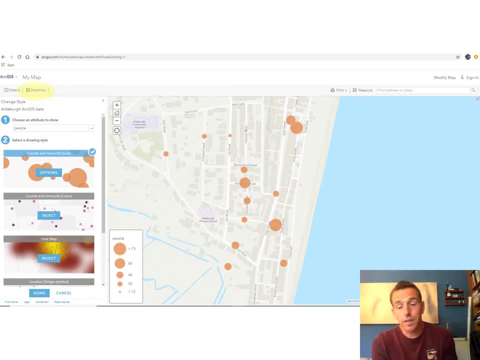 really good to things like pollution levels or environmental quality or things like flood risk. even So, once you've got the data in there, you can play around and make this map completely bespoke to you. The other things that you can do is you can change the base map. 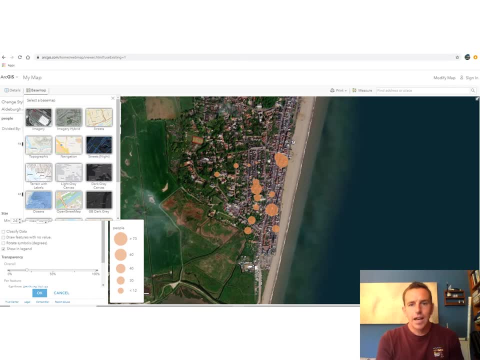 you can make those symbols bigger or smaller and ultimately you can really be creative in making this map, which is also a form of presentation. it's not just a map. it's now a map with data on it, and therefore we've classed that as a piece of gis, and you then got that to use in your 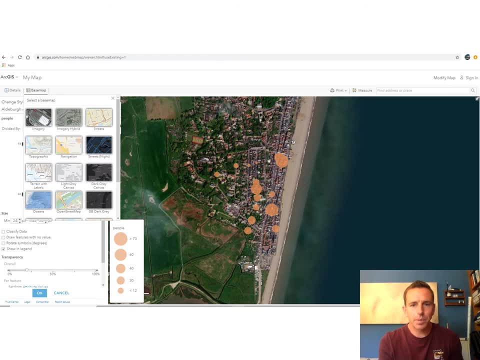 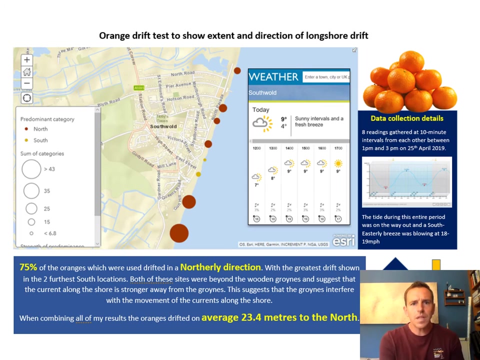 nea. so what we normally encourage students to do is that when they've completed, fiddled and tweaked their map, that they screenshot it, they crop it and they paste it into a word document and then it's then very easy to add other things on to that map that they've created. so this one. 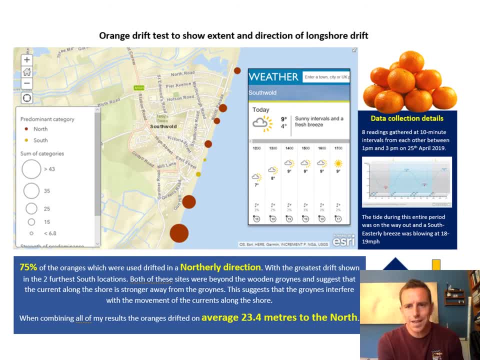 here. we've often asked this question about doing longshore drift tests. what's a good way of presenting longshore drift data? well, again, it's up to you how you do it, but we came across this example that a student did a few years ago and i thought it was brilliant, really creative way. 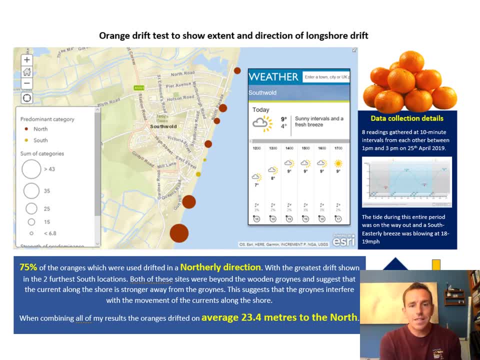 of presenting longshore drift data, and it's a really good way of presenting longshore drift data and what they did, rather than using a line graph or a pie chart or anything like that. they gathered their data and then they worked out the velocity, the average velocity that the 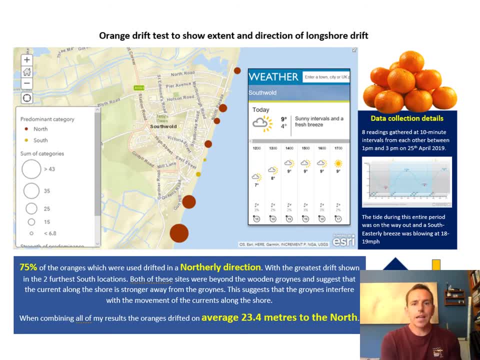 orange traveled at each location that they did their longshore drift test and they also had the latitude and longitude for each location where they threw those oranges into the sea. and so in their excel document they typed in their latitude and longitude and then the third column was to represent the average velocity that the orange was traveling, and you can see. 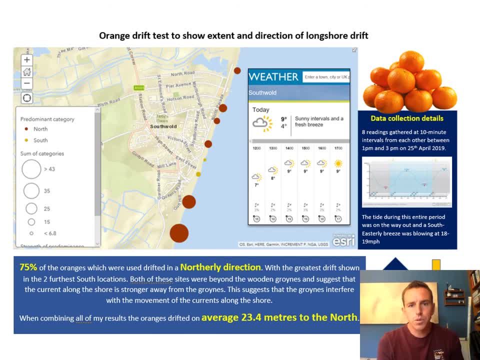 here that that student has then got symbols representing how fast the orange traveled. that's shown by how big the orange is. and then the other thing that they were also able to do was to have two different sets of data. one was to show oranges that moved in the northerly direction. 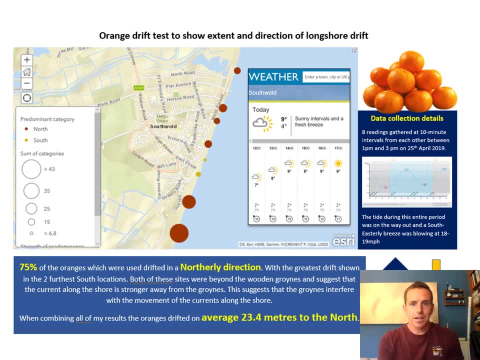 and one was to show oranges that moved in the southerly direction, and so that's why there's two colors on that and that's an- again a very interesting way of presenting longshore drift data. So they were then able to take a screenshot of that image and paste it into a word document. 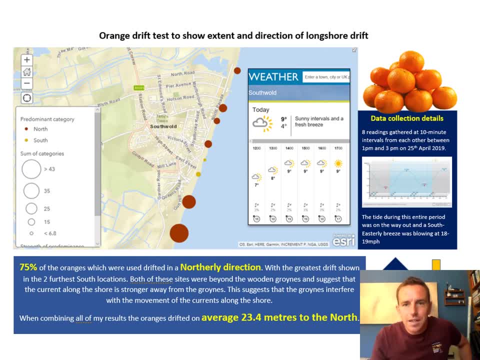 added an appropriate title and remember earlier I said: make sure you're considering or you're including a recognition of the external factors that may have influenced your field work. so for something like an orange drift test, it's then also been appropriate for this student to include the 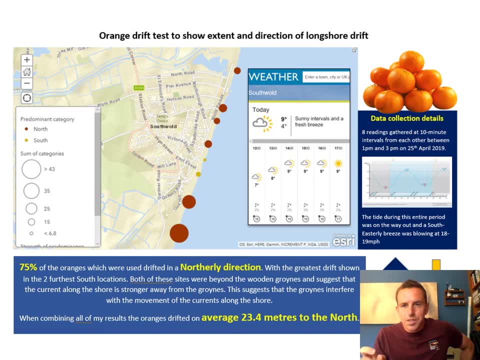 weather conditions on the day and also a recognition of what the state of the tide was on the day while they're doing their field work. so you've got two extra bits of secondary data there. essentially, that has been added onto this bit of primary data. it's GIS. it's got a bit of analysis with some data interpretation underneath that as well. 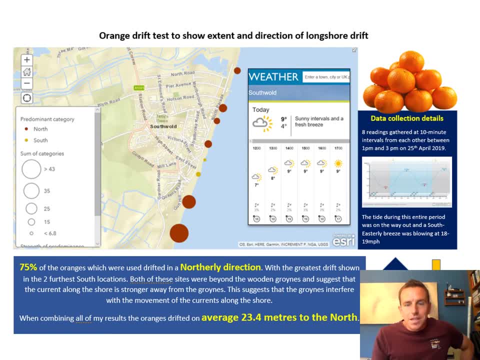 that, in my opinion, is a really, really nice way of presenting modern field work data, and if you compare that to a line graph or a pie chart, and it's completely black and white. this is so much, and that is something that you guys can do. Key, then, is making sure that you have got. 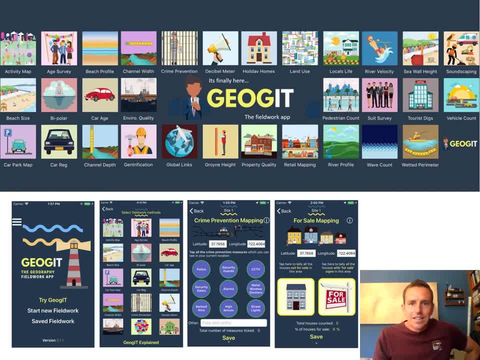 latitude and longitude with the data that you collect. so this is something that we, a few years ago, were quite passionate about in terms of trying to modernize. we were, you know, wanting to move away from this idea that field work is all about clipboards and paper booklets. 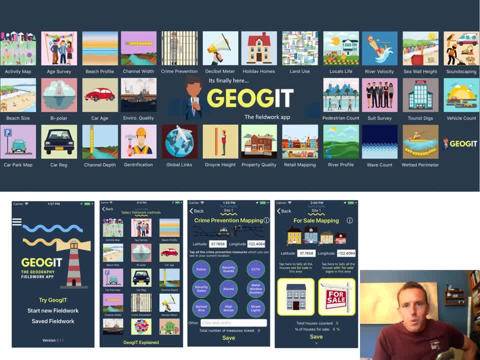 and kept on looking at our phones, thinking there's got to be a better way of collecting fieldwork data, and there absolutely is. and at the moment we underutilize our phones and I think it's about time that we've started to embrace those and to use more modern technology. 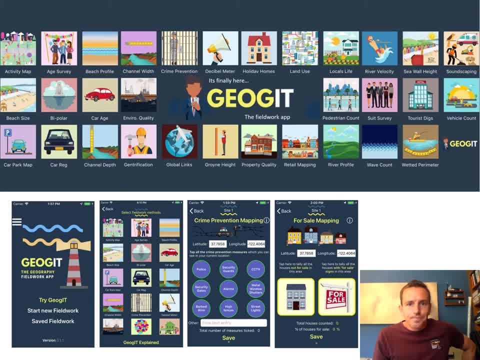 to gather our data, to make data presentation easier. so the principal idea of Jogit, the fieldwork app, was to enable students to geolocate their data by automatically tagging their data that they collect with the latitude and longitude coordinates. so all the data you gather using Jogit has got the latitude and longitude coordinates automatically stamped on it. 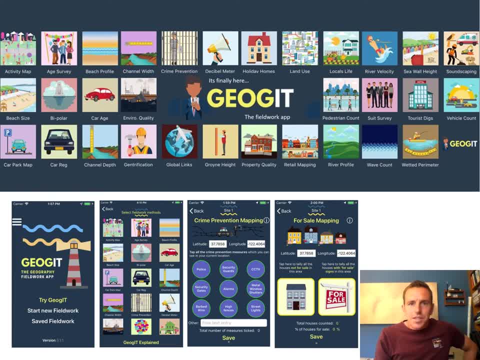 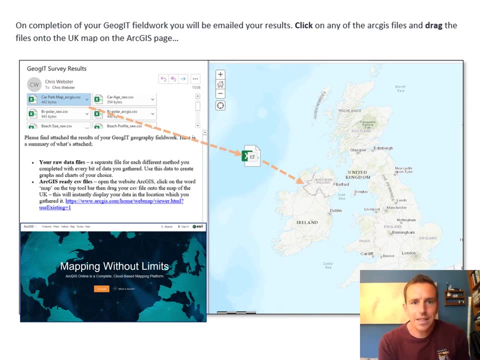 what happens with Jogit when you're collecting your data is that, behind the scenes, these excel spreadsheets that I showed you are gathered for you and are built for you as you're logging your data. ultimately, what you're able to do with those files, then, is you are sent them automatically upon. 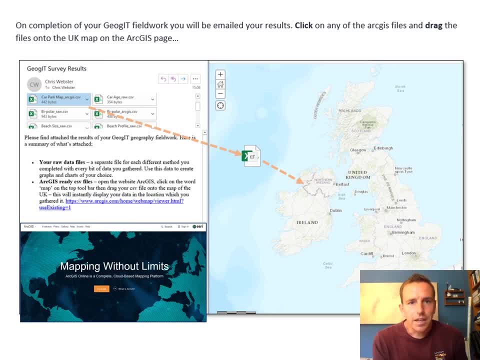 completion of your fieldwork, you get an email that looks like this. it says: thank you for using Jogit your data. that data is automatically and already complete and organized in excel format. you're then simply able to drag those files that arrive in your inbox into ArcGIS and straight away. 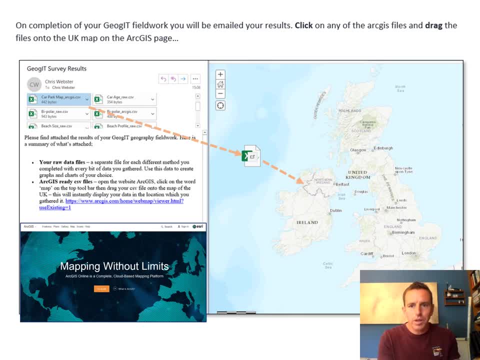 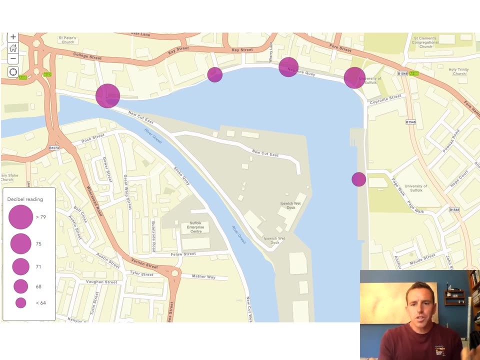 without any data input and having to go through soggy booklets and transferring data that you can't really recognize onto the computer. it's already done for you and it is then able for you to then manipulate and to interpret and to and present in the forms that you want. so Jogit just makes the most of the technology that you. 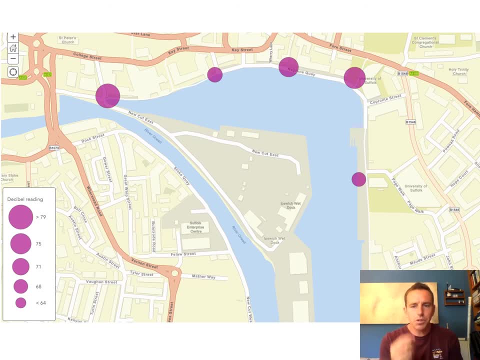 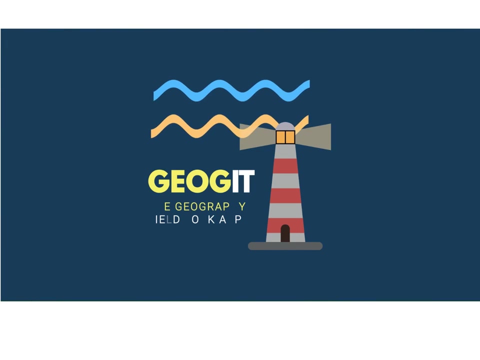 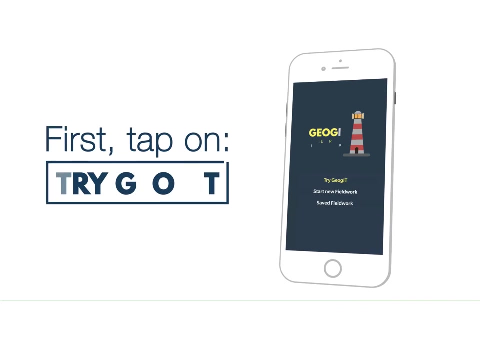 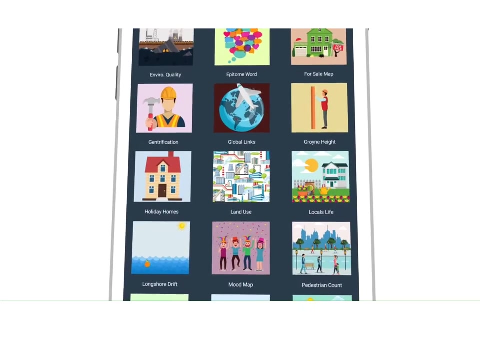 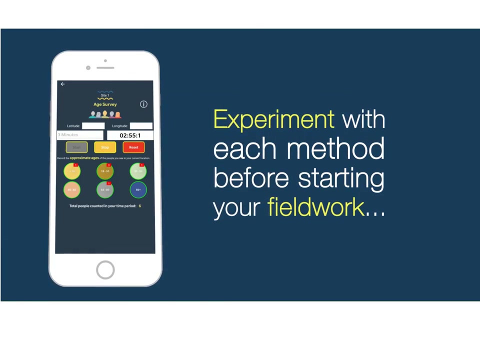 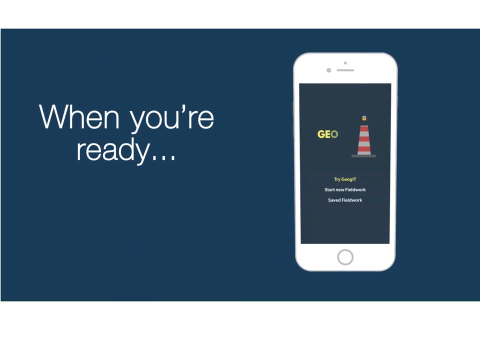 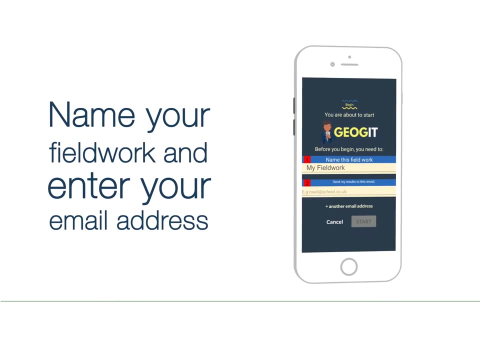 have to make your data better by geostamping or geolocating it and enabling you then to instantly transfer it into ArcGIS without having to manually data input, the data that you've got, and then going back to the Jogit way, way, way way. 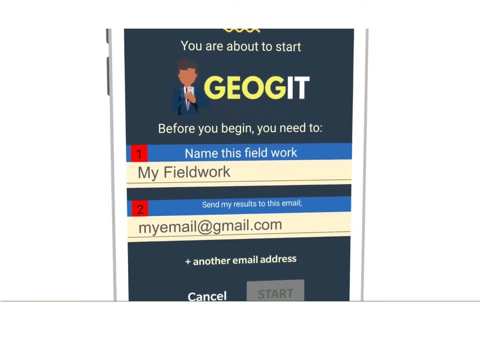 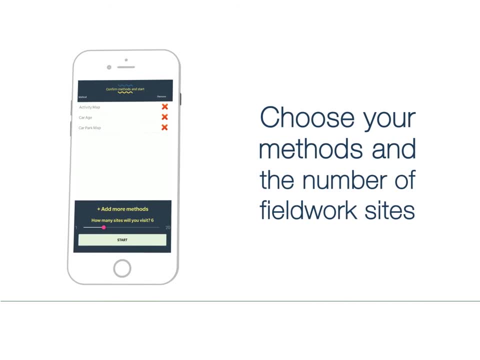 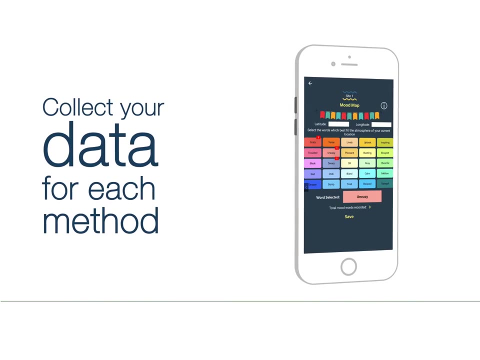 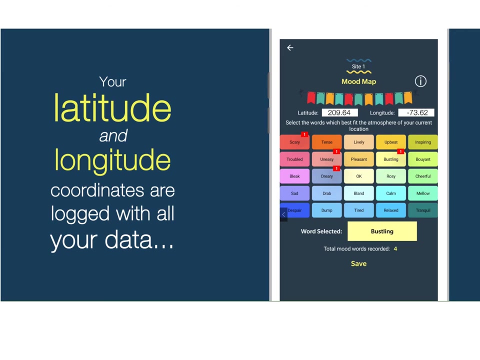 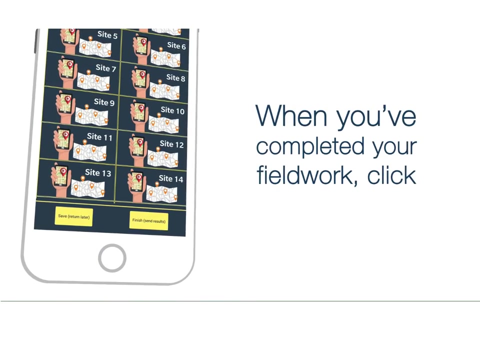 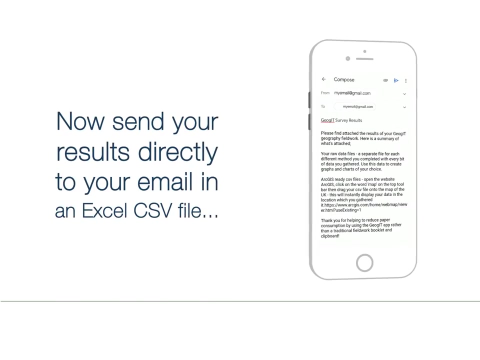 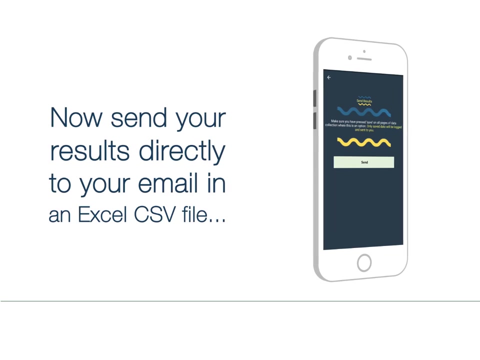 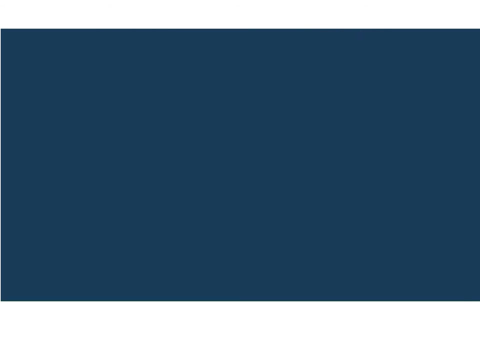 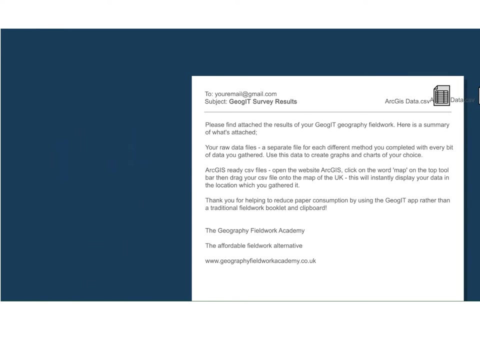 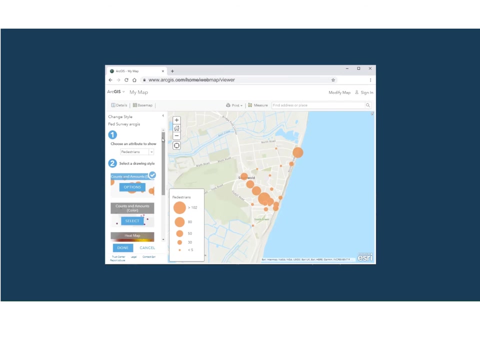 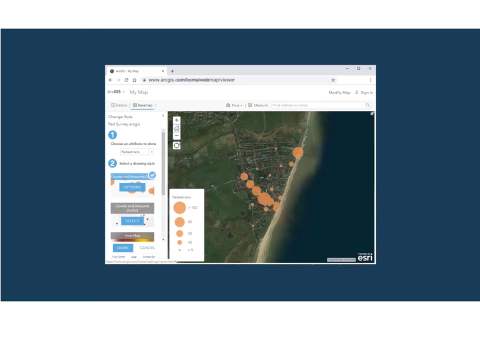 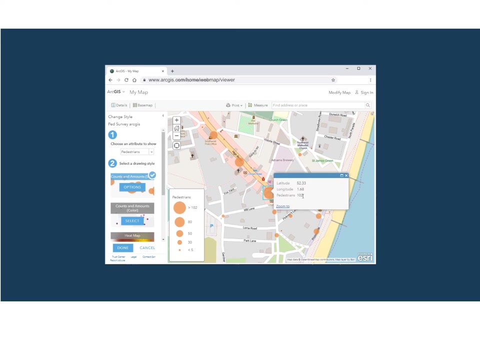 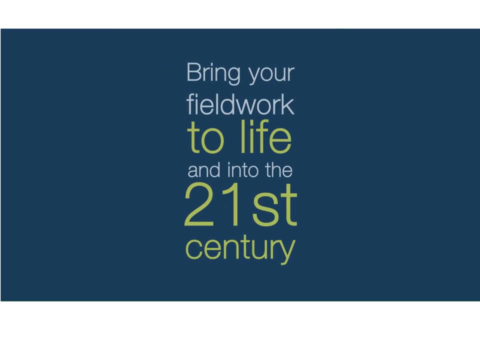 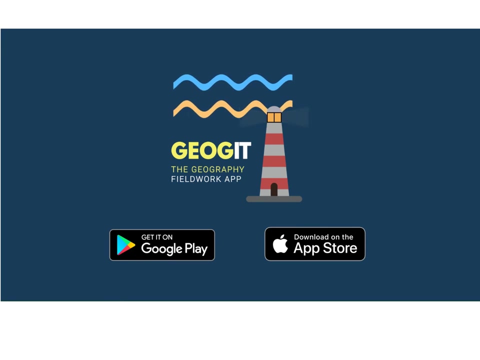 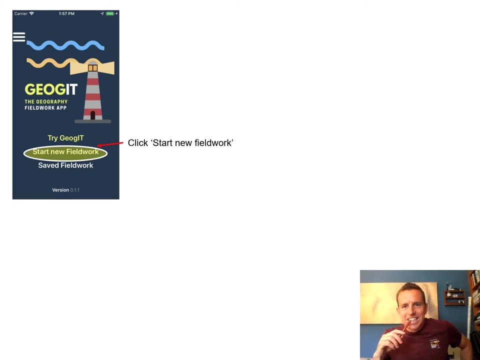 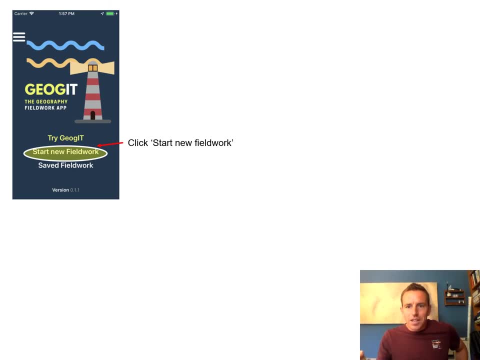 last year And we will acknowledge that on Jogit, there are some methods that have the criteria on it fixed and therefore it's not necessarily completely appropriate at any A-level to be using those with fixed criteria. And it might well be that you look at some of those methods. 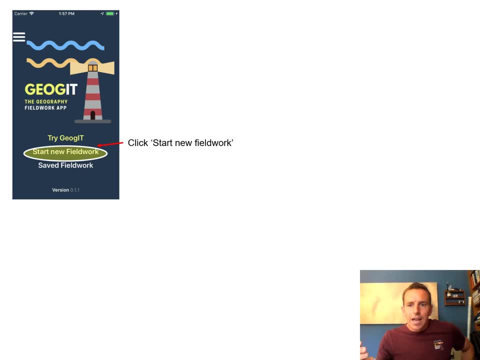 and you just gain a bit of an idea or inspiration from them and then you create your own. You make your own bespoke method from that. But actually about 25 of the 35 methods are completely appropriate to use and they don't have set. 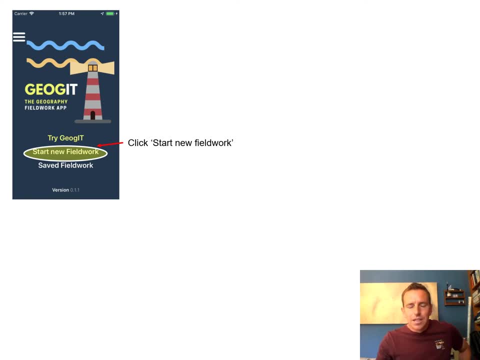 criteria And essentially, they're just counters, And they're counters that enable you to complete a number of different surveys, whether they're river-based, coastal-based or urban-based. So I'm just going to talk through how you go about using Jogit. 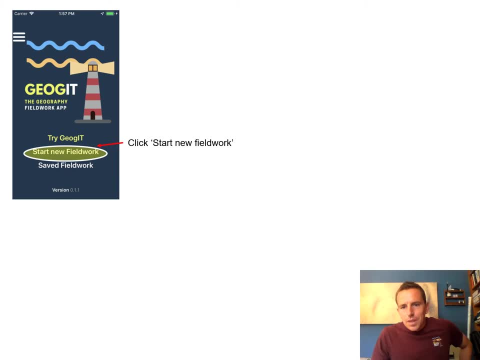 It's pretty self-explanatory, but I'll go through some of the basics with you. So when you have the app downloaded and you can get it off the Apple Store or the Google Android Store, this will be the first page that comes up. 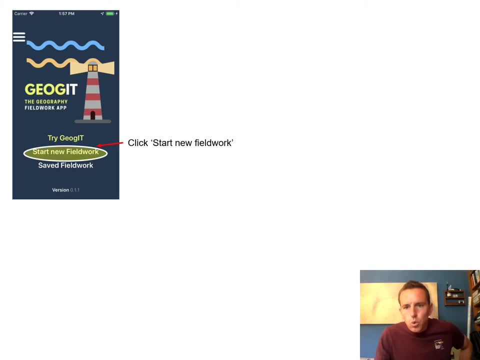 after a brief introduction, And so this is your home page for Jogit. If you wanted to, you could click on the top one there that says Try Jogit, and you can just explore the different methods that you can do and just see what the app offers. 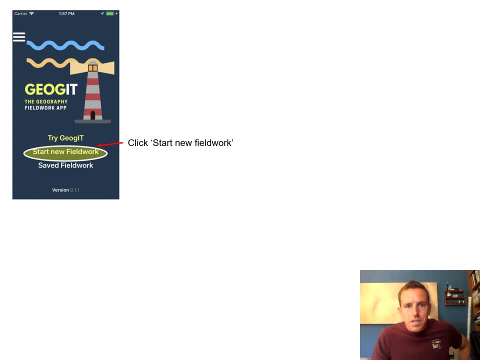 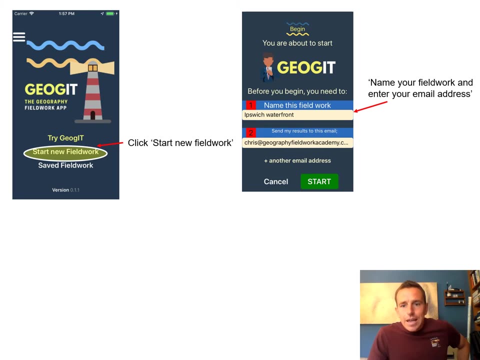 But when you're actually ready and you've got the experience of what ones you're going to use, click on Start New Fieldwork. When you've done that, it will prompt you to enter in your name for this fieldwork, So it might be. 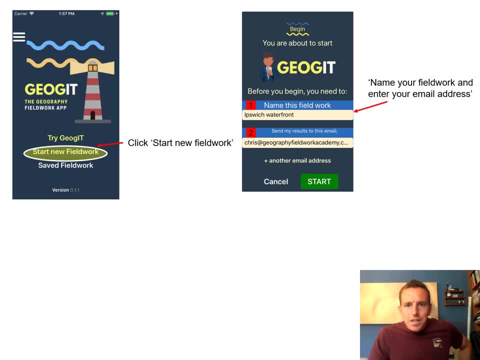 NEA Data Collection Day. 1. Enter in your email address. This needs to be an email address that you can access, So if it's a school one or a work one, then make sure that you've got access to it when you need to, So at home. 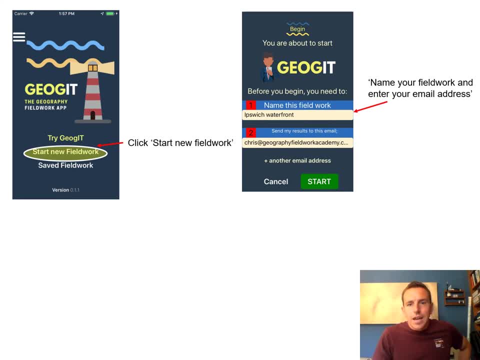 if you're planning to do your data presentation at home, So you can actually add in a couple of email addresses there. It might be that your teacher wants a copy of your fieldwork, So you can add in as many as you want there Once you've added in. 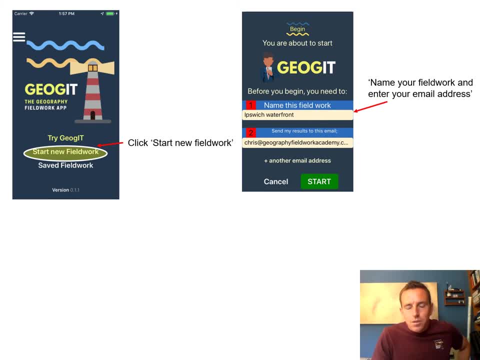 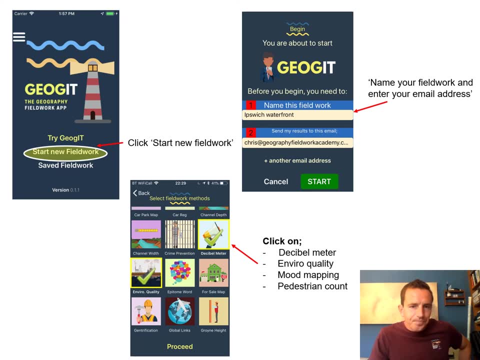 a valid email address, the Start button will turn from grey to green. That means you can select that button. That then allows you to proceed onto this page here. This page is a scrollable page that you're able to go up and down on And simply you just need. 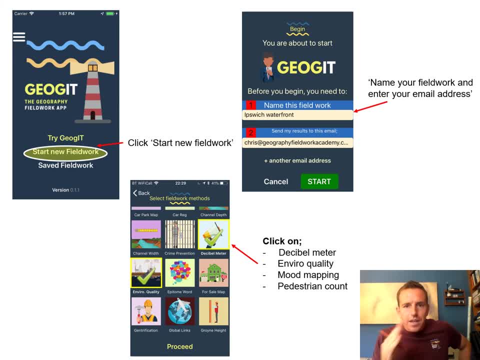 to tap on the methods that you are intending to use on that day, And they will then be built into your electronic fieldwork booklet So you can tap on as many as you want. Then, on the next screen, it will tell you which methods that you've. 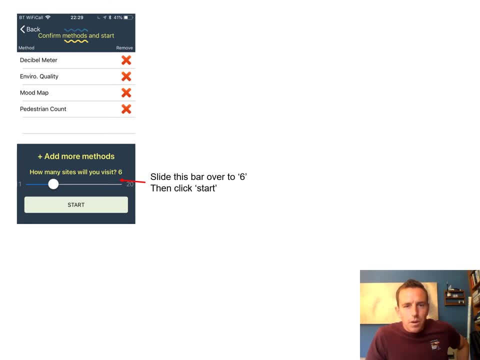 selected, And if you've accidentally selected one that you don't want, you can delete that there. If you want to go back at this stage and add another one, you can do by clicking the Back button on the top left And then once. 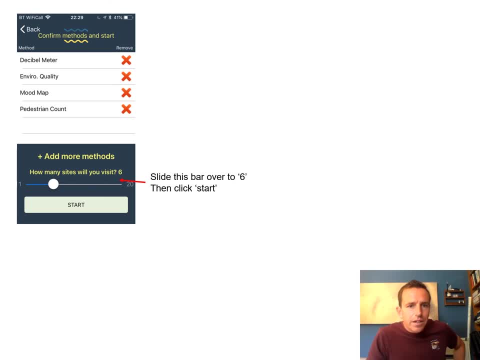 you've done that. just slide that slider along there to say how many sites you're going to visit. It's probably a good idea to go higher than lower. So if you're not quite sure how many sites you're going to visit, then just slide it all the way across. 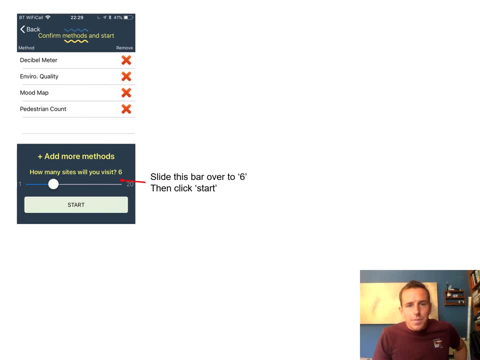 to 20.. And that will enable you then to visit as many sites as you want. And if you don't visit all 20 sites, then it's absolutely fine. It will just send the data from the sites that you have been to Again once. 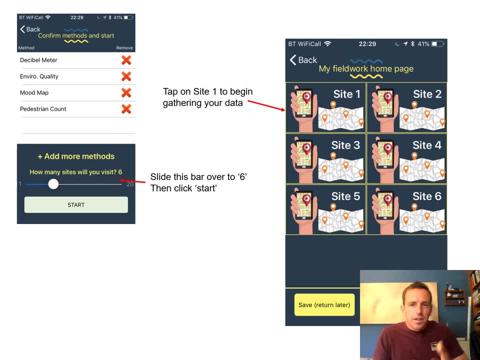 you've done that, click Start, And that then takes you to your own fieldwork home page. The idea of this, then, is that you have a different- almost like an advent calendar, really. you have a different window for each of the sites that you have. 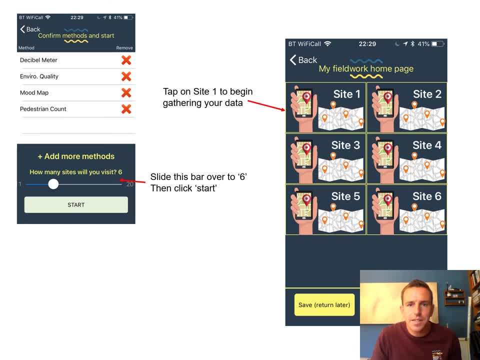 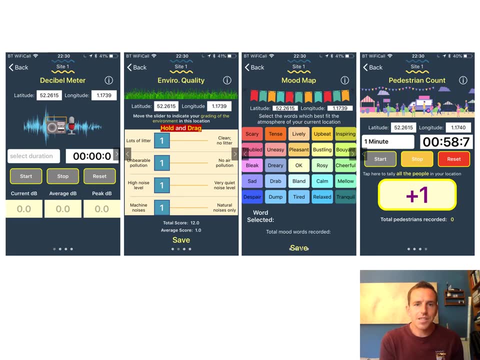 suggested that you're going to visit By clicking on one of those sites. it will then take you to your first method and then you'll be able to swipe left and right at that stage, to the other methods that you have selected. And once you're in this zone, then you 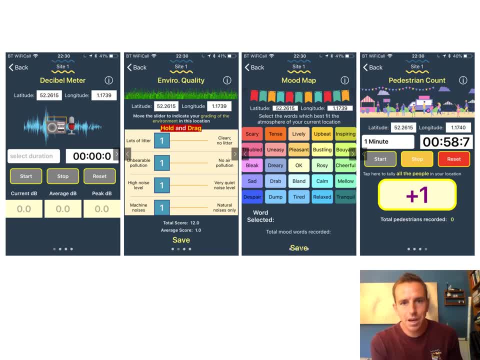 can see that the latitude and longitude comes up And you can then start gathering your data. Where there is a Save button at the bottom of those fieldwork pages, click that when you've finished and that will then just make sure that that data is logged On. some of them that are: 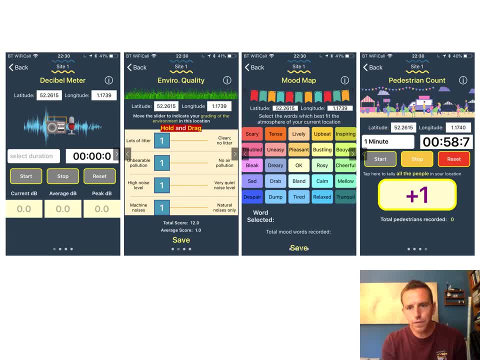 timer-based. you don't need to click Save because when the clock finishes, it automatically saves the data for you. There are things like a mood meter and environmental quality survey that you've got there. It might be that you intend to come back to that and 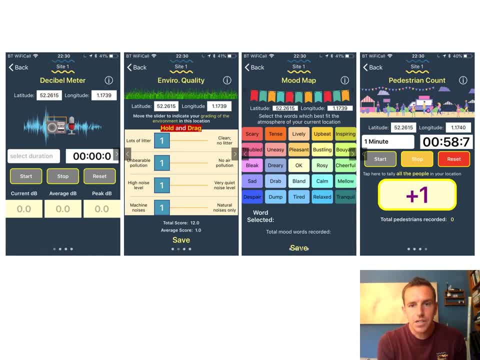 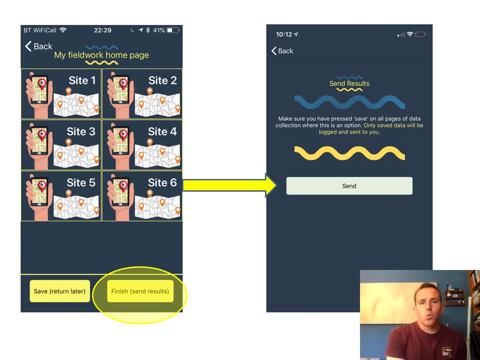 amend it. So just click Save when you have finished it, and then that will mean that that's then virtually kind of sent off and it's logged Eventually. then, when you've completed all of the fieldwork that you intend to do, it might be that you've visited four of your. 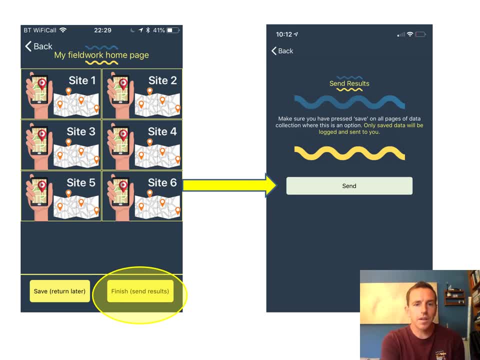 six sites or that you have gone to all six sites and you've done everything that you want to at those six sites. You then need to click on Finish and Send Results. This will then come up with this next page and generate this next page where it says Send Results. 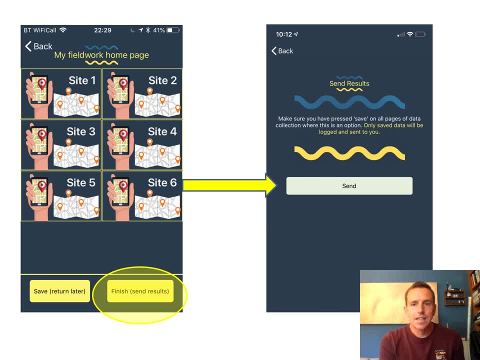 And you then simply need to click on Send, and an email then will be composed to you with your results attached to it. You'll then be able to access that from your inbox. drag your data into ArcGIS, and instantly you'll be able to start creating. 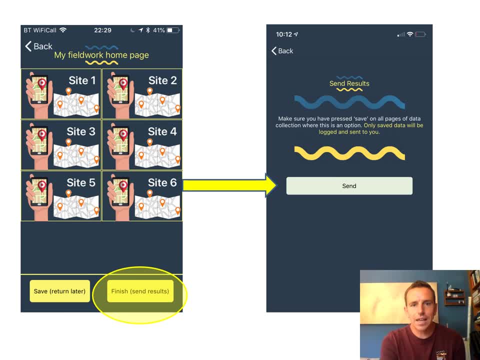 really high-level, modern pieces of data collection. Just at this point it's well worth me just saying that if you get to this point here where it says Send Results and that Send button for any reason isn't there or is kind of greyed out, 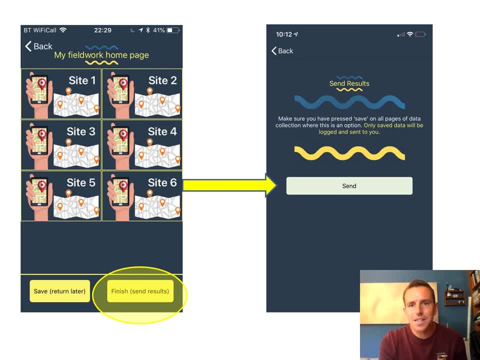 then 99 times out of 100, what this means is that you haven't got Apple Mail downloaded on your iPhone, So this is normally only an issue of iPhones. Sometimes it might be an issue of Android, and it just means that you need to. 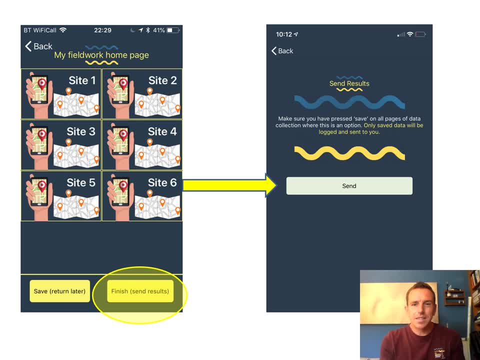 sort out or need to download Apple Mail. That is the default email system that Jogit uses to send results. So if you have any issues at this stage where your results are not being able to be sent, I can normally guarantee that the main issue at this point. 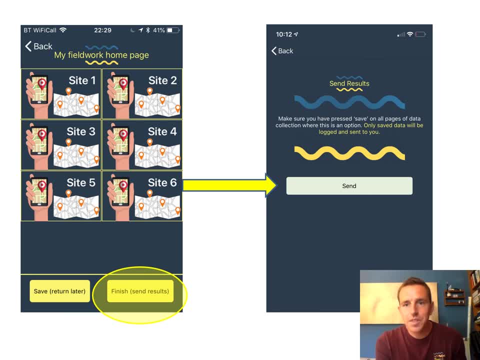 is that it's because you haven't got the email system downloaded onto your phone. If you do have issues with Jogit, then there is a link on Jogit to access our support and just send a message and we will be able to get back to you. 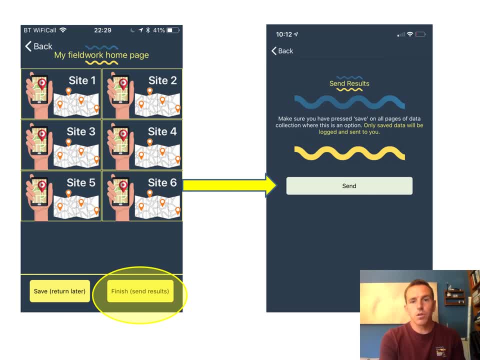 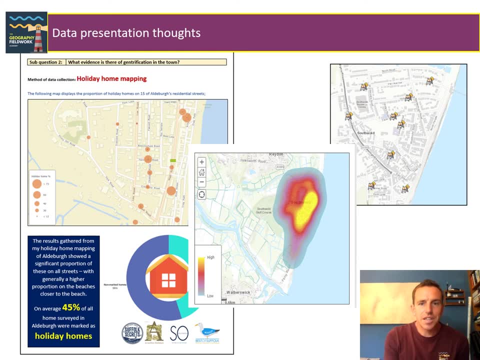 To just give you a bit of support as to resolving that situation. Okay, so the reason that, as we've said, Jogit and using ArcGIS is really useful is because it allows you to present and create really nice colourful, modern, engaging pieces of data presentation. 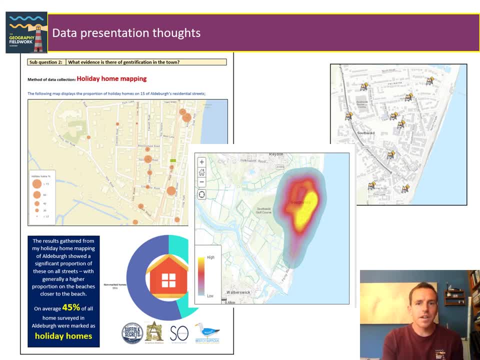 And again, these are completely up to you to customise and to make bespoke. and as you play around with ArcGIS, you'll see that there's lots of ways of creating really lovely visual pieces of data presentation. There's lots of videos that have been made. 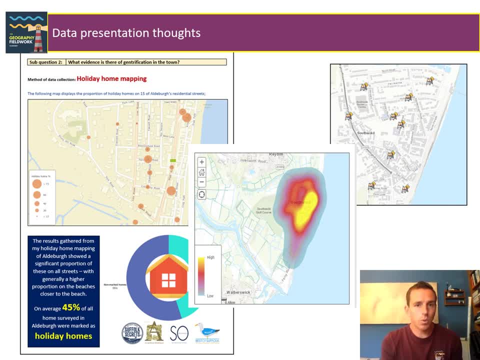 from ArcGIS that are available on YouTube, and their support team is fantastic as well at helping you out with other things that you can do. I have essentially just kind of touched upon the basics here. There will be many of you that are much more technically. 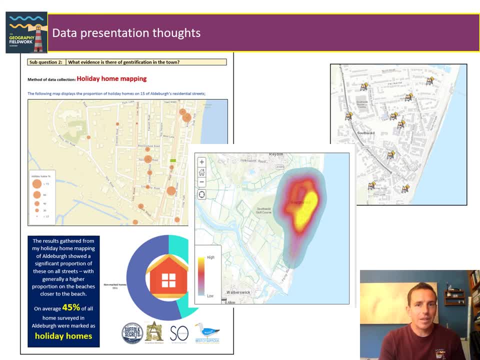 gifted than me and will be able to very quickly become experts at ArcGIS and the things that you're able to present on it. So explore it. if you've got the time and the creativity, explore that website to make the most of the data that you've got. 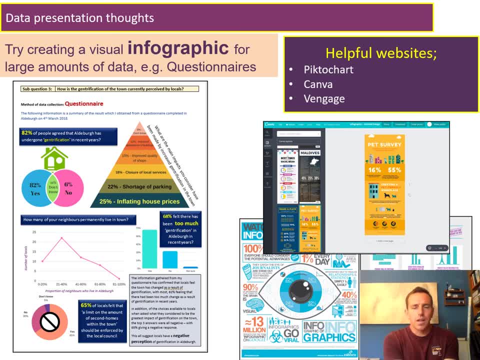 Last thing that I'm going to just touch upon. I'm not going to go through a huge range of ideas for data presentation because, again, this is something that is independent to you and it should be your own thoughts and your own research and ideas that are generating the ways in which you think. 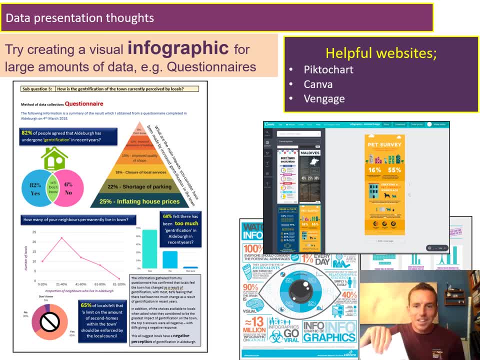 you're going to present your data. Having said that, I would again suggest that this document, the ArcGIS NEA Guide, is well worth having a look at, because it has got quite a lot of traditional forms of data presentation, which is still really appropriate, but 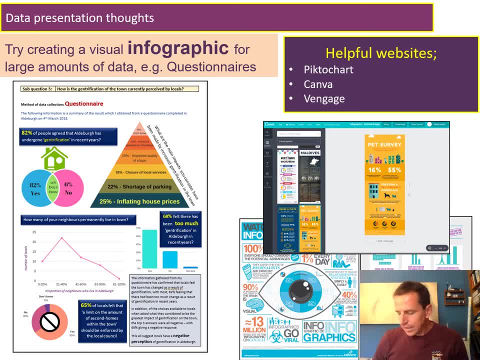 it has got a lot of good ideas about how you can present your data in relevant and appropriate, suitable formats, But one of the things that I thought I'd just mention is that we very often get asked by students: how can you present questionnaire data in a more engaging way? 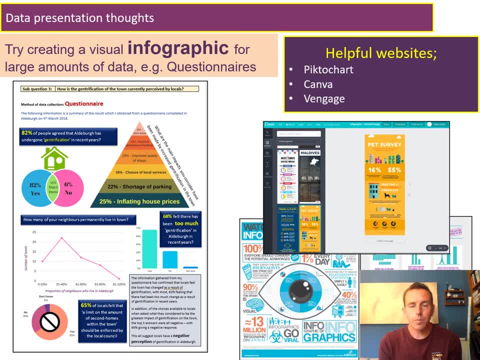 And one of the things that are more readily available for free nowadays on the internet are these infographic free indicators, And we generally use the website there called Canva, for creating a lot of our marketing and social media posts and literature and brochures and stuff like that. 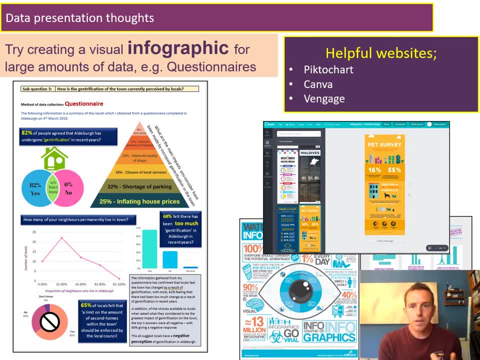 and these websites give you the opportunity to make bespoke pieces of data presentation in formats that are perhaps more engaging and different to your classic pie charts and bar graphs. So, again, you can play around with the templates that are available here and you'll very quickly become confident. 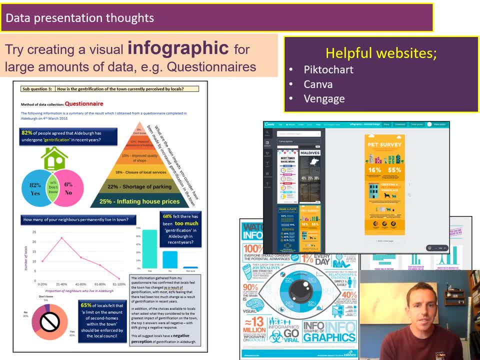 in using them- Changing the fonts, the colours, the sizes, the scales, all sorts of things like that- And an infographic then is where you try to present a range of data in a more creative way, and they're becoming very popular with marketing companies. 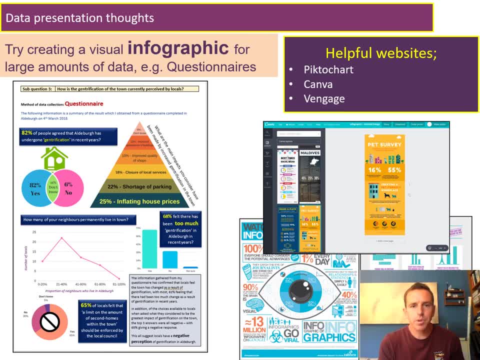 and you'll see in most magazines now many adverts are presented in an infographic format, And it's a good way of presenting lots of data in a more creative visual way. So have a look at perhaps how you might be able to use those in your survey. 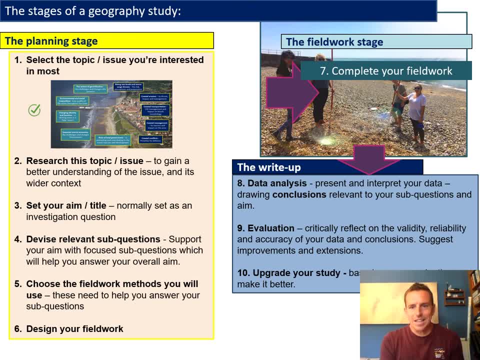 Okay, so we are pretty much getting there, And the idea of these six videos was to help you with the planning stage of your NEA, which is a challenge. It's something that you guys have not experienced. that because it's now no longer. 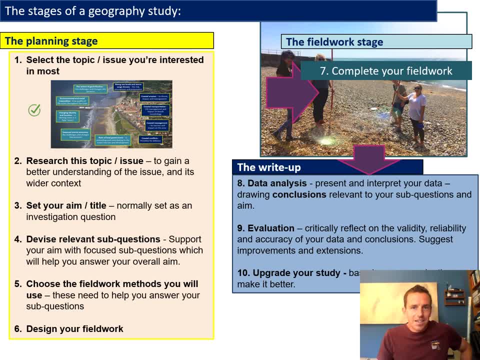 part of the GCSE. So planning a NEA is a considerable challenge But it's something that hopefully you do now feel a bit more confident with. We've gone through that bit on the left there, that yellow box, We've kind of picked. 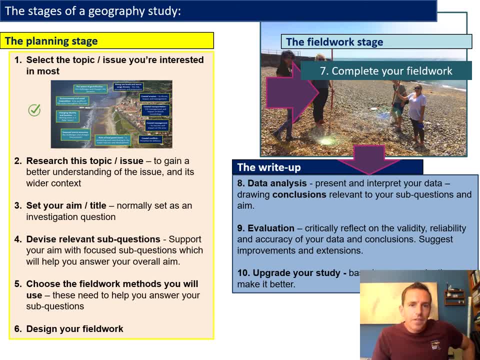 out all of those things and others, And we have covered the things that you'll need to be aware of when you're planning your NEA. You can go back over any of these videos, obviously, and, just you know, recover the things that I have. 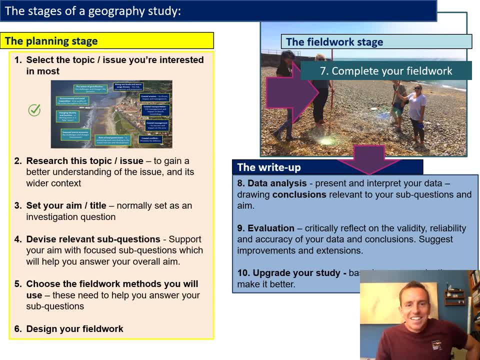 perhaps talked about. There might be some things that you skipped through. I don't blame you if you did, But we have covered the key aspects of the things that you will need to think about when planning an NEA And essentially, now it is up to you. 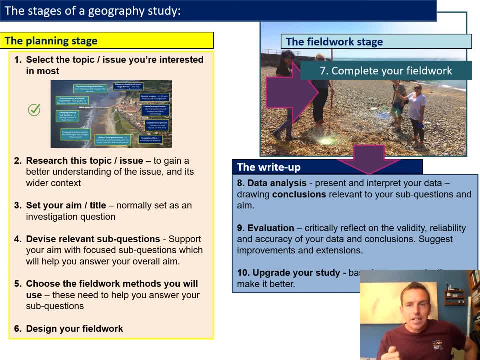 to use that information, to speak with your teachers and to consider what fieldwork it is that you're going to do, And then to go out and do it. And again, as I said a few times before, don't worry if it's not perfect Fieldwork. 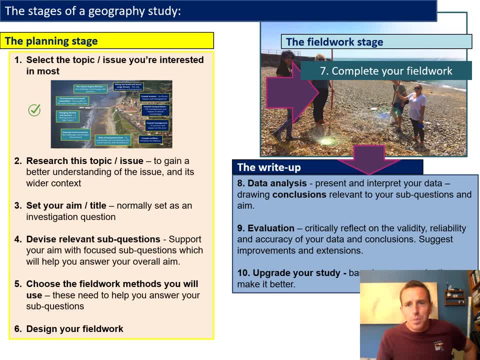 doesn't have to be perfect. You can tweak it, you can amend it, But if it's not perfect, it's fine And you can write about that in your evaluation. So the big bit, the write-up bit again, is something that you'll. 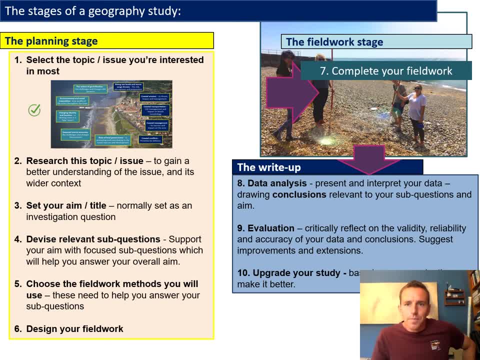 need to think about with your teachers And I'm sure they will give you some input as to how you perhaps might tackle that. But again, that is largely independent. There will need to be your own work and down to you as to how you structure it and the kind of things that you focus. 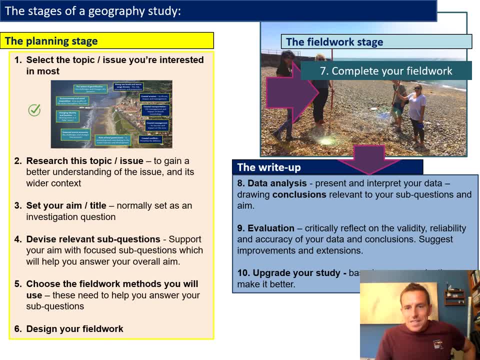 on. But the key thing from our perspective- particularly this year, when it's difficult to access not only the support of your teachers, but perhaps fieldwork tutors as well- the key thing that we wanted to do was to help you get started on the right footing. 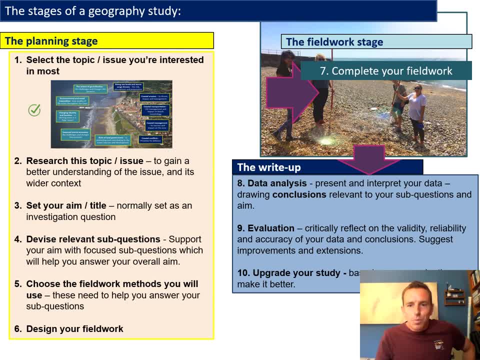 And if you do that, it's fairer, I think, And it enables you to then write a better NEA, prepare and plan and conduct a better NEA, and you're then in a better position to do yourself justice for this part of the Geography course. 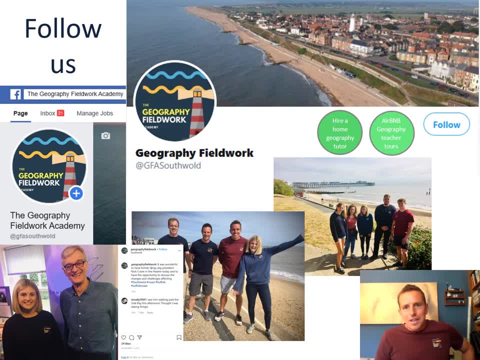 So that's about it from us. What I would say is that if you do need to access support for JogIT, or if you do just want to ask a general fieldwork question, we're not as busy at the moment as we normally would be, unfortunately. 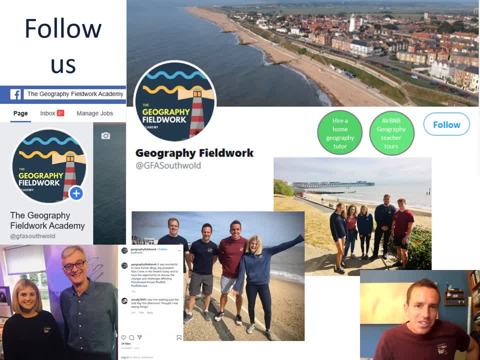 And so we do have more time on our hands to reply to any questions that you might have, so don't be afraid to give us a message. We're on obviously all the normal ones: Instagram, Twitter, Facebook, stuff like that. We've obviously got our videos uploaded. 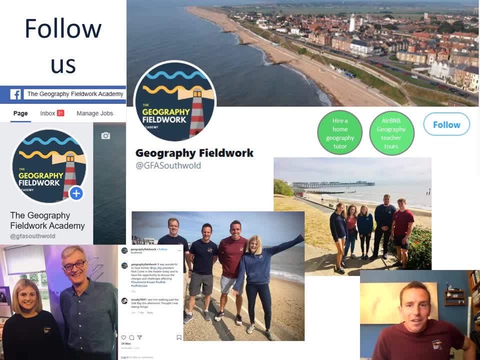 onto YouTube A couple of other things that I'm going to shamelessly plug. We've had to adapt, like lots of businesses this year, to the changes that are happening in our country and around the world, And one of the things that we're determined to do is to be 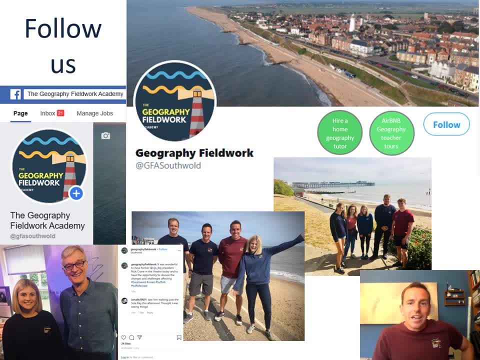 here next year and to keep going and to keep growing, And so we've had to think about how fieldwork will look going forward and how we as a business will look going forward. So there's a number of things that we're working on. We're starting to work. 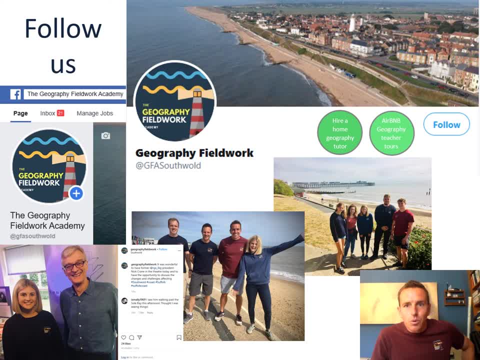 with the local national park here in Norfolk on a project over the next few months. But we're also working with Airbnb to deliver geography experience tours of Southwold. So if you are in Suffolk over the next few months, then look those up and we would be delighted to give you a. 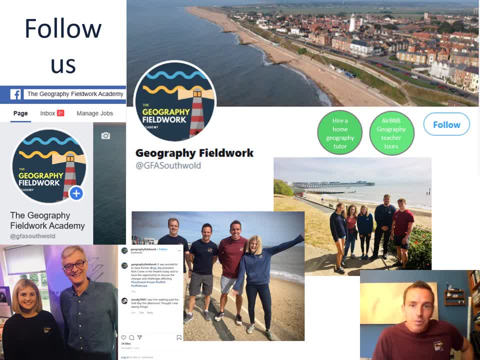 personalised geography tour of Southwold. But the other thing which may be of more interest to you, or maybe somebody that you know, is that over the course of this year and perhaps going forward, we're going to be providing a bespoke hire- a home geography tutor service. 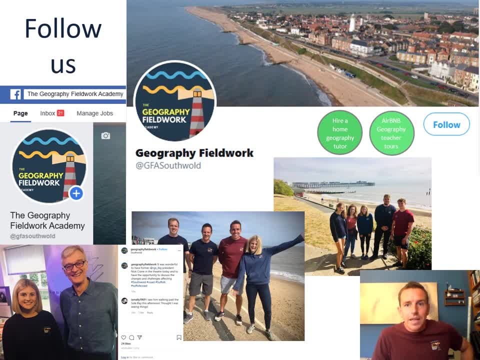 So we have all probably become familiar with things like Microsoft Teams and Zoom over the last few months And we've realised that this is a way in which we could actually offer another opportunity to students and we could support students virtually by giving geography tutorial support. 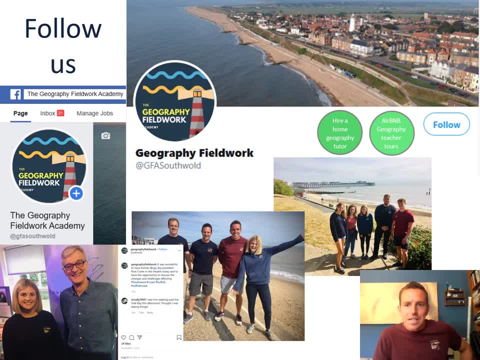 Myself and my colleagues have taught geography at GCSE and at A Level. We've marked NEAs at A Level as well, And so we are in a strong position to be able to give you support if you need it And over the course of this next year. 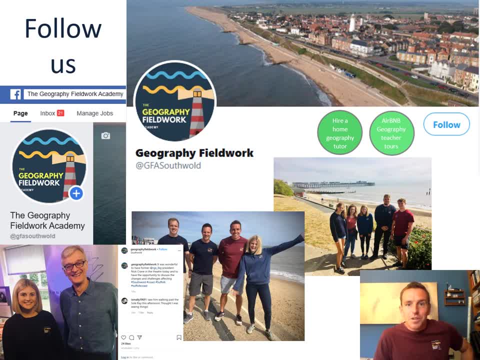 there may well be a number of people who feel like that. they perhaps do need a bit more support, And so, on our website, if you click on that button, you'll be able to go through to a page to contact us to submit your enquiry about having access to a geography. 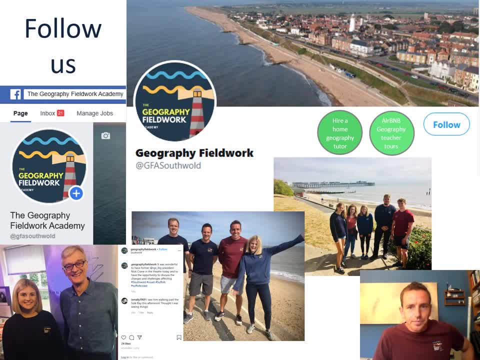 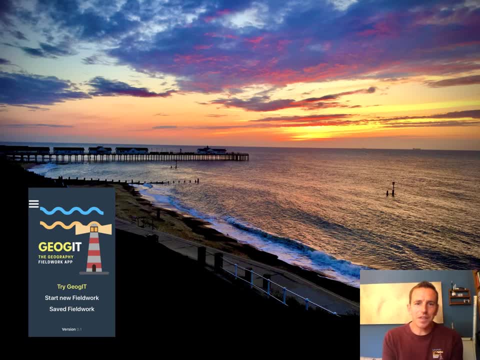 home tutor, So it's something that we'd be delighted to help you with, Okay, Finally, then, we want to wish you all the best with your NEA, and we're pretty confident that you have got all the tools that you need to start planning and conducting. 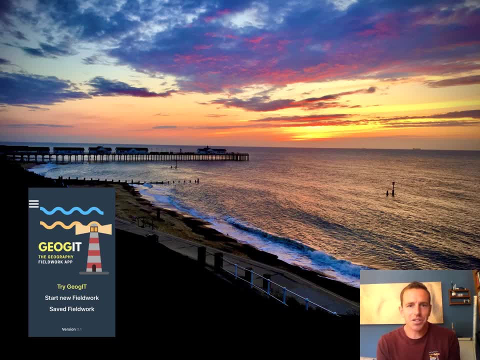 a really top quality independent investigation. We've done these sessions for free and we're delighted to do that. It's our job to support students in fieldwork and it's our pleasure to be able to do that, even at the moment when it's not physically possible for us to. 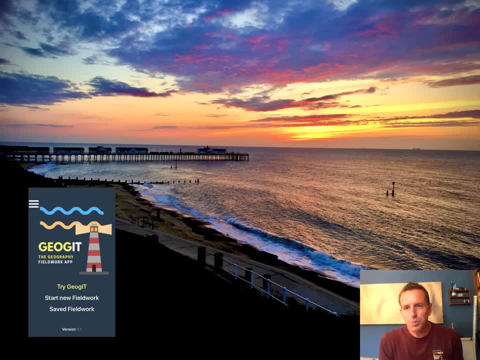 be delivering our courses, But the one thing that we would ask if it's possible for you guys to do to help support us, just to add a little bit of a contribution to our coffers, is to go on to the Apple Store or the Android Store and 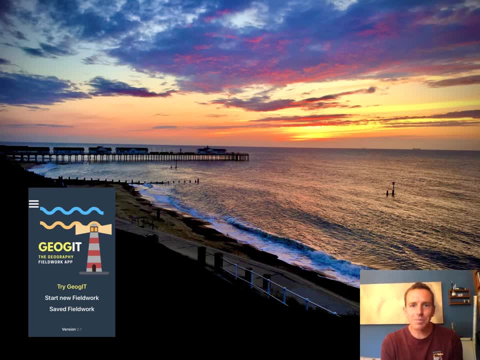 download Jogit. We get about 70p for every 99p download. That might not sound like a lot, but every little helps and that will help us over the next coming months, just to continue to keep going, to keep supporting teachers and students and hopefully. 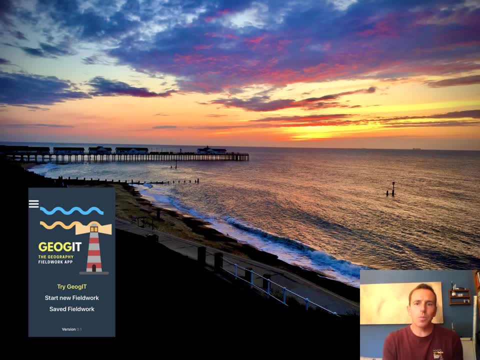 when things start to improve, to be here to help deliver fieldwork in Southwold into the future and beyond. Once again, good luck with your NEAs and hopefully see you in Southwold one day soon. 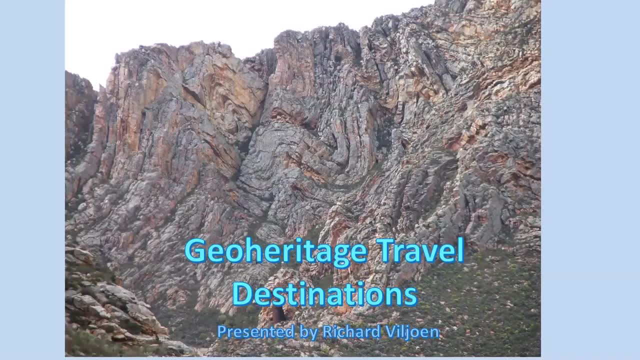 Sound okay. Welcome to this afternoon's lunchtime lockdown lecture, which is by a trio of people- Richard and Morris Villioun and Alan Roxton Wiggle, on geoheritage travel destinations in South Africa. A big thanks to Tacoma Strategies for sponsoring the month of September Without. 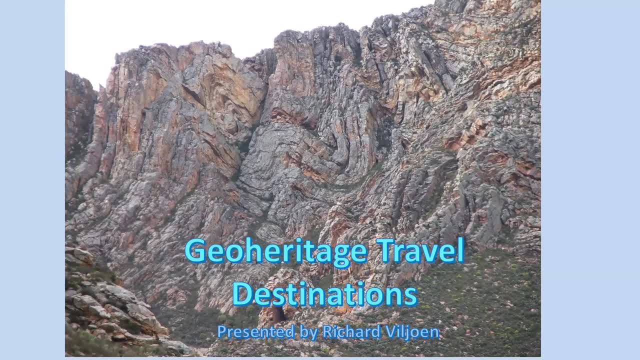 the sponsorship. we couldn't run these things very easily, So thank you very much to Tacoma and Matt Mullins. Before we start, we will put this presentation onto the GSSA YouTube video channel, But you're reminded if you download or use any slides from the presentation, please. 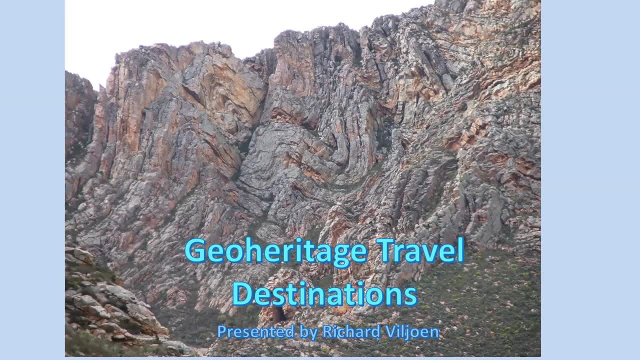 make sure that you give proper credit to and recognition to who it's due to. This afternoon's presentation is going to be a three-part. First up is Richard, second is Morris, third is Alan, And I think Richard and Morris need very, very little introduction, So I'm going to. 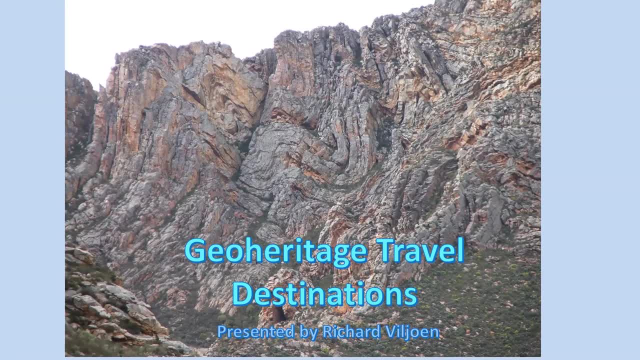 refer you to the blurb on the Google calendar. I think we all know who they are. Alan is relatively new to the geoheritage family in South Africa. He is the CEO of something called geoheritagetech, And he is in fact a geologist but practices more as a geotourism guru, I think. 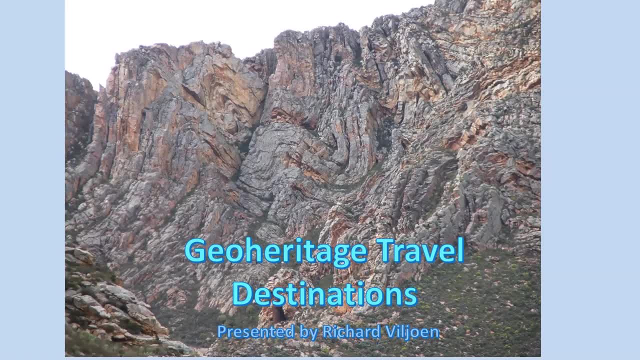 that's probably enough said, And with that, Richard, I think you can take it away. Thanks, Craig, And good afternoon everyone, And thanks for your participation in this event. We would like to thank the organizers for making a slot available for us in this geoheritage series. 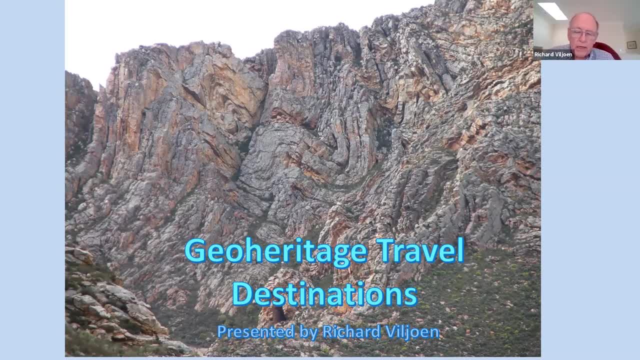 which I think has been a great success, And pretty interesting to hear what's happening with in geoheritage in South Africa, particularly for the generations to come. with 25% of them serving tutors, That's pretty racing as well, And you know it's thissten ahead of time.